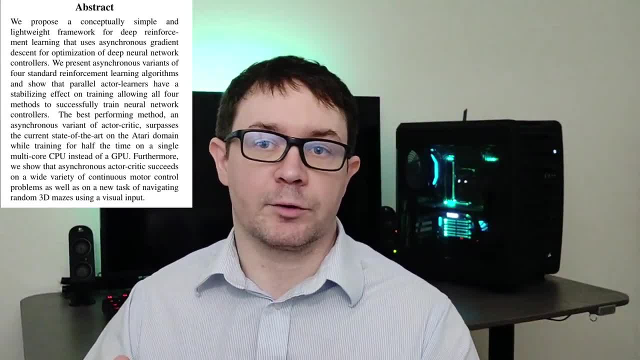 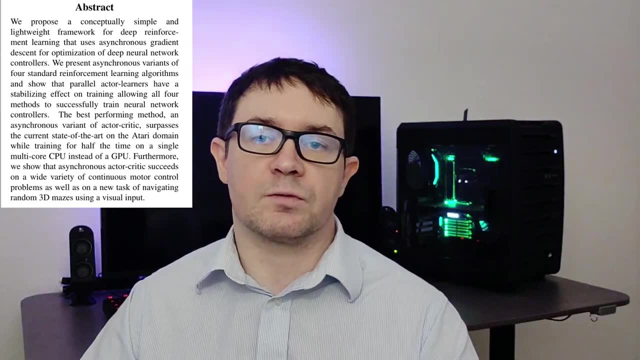 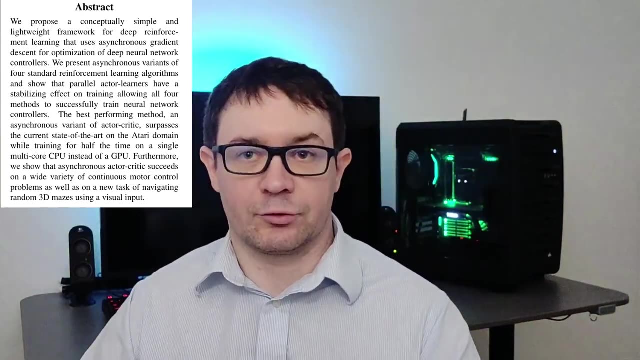 It's a totally different paradigm for approaching the deep reinforcement learning problem and in fact the technology can be applied to a wide variety of algorithms. In the original paper they detail solutions for deep Q-learning, N-step Q-learning, as well as SARSA and actor-critic methods as well. 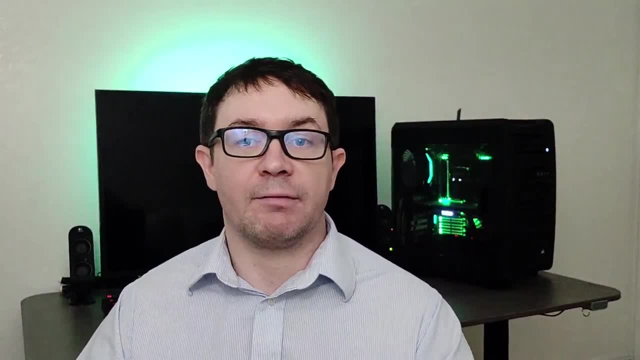 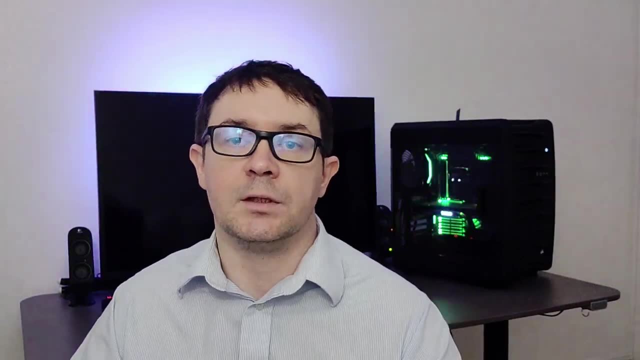 So what is this big innovation? Well, instead of having a replay buffer, we're going to allow a large number of agents to play independently on totally separate and self-contained environments. Each of these environments will look different. Each agent will live on a CPU thread, in contrast to a GPU. for most deep Q-learning applications, 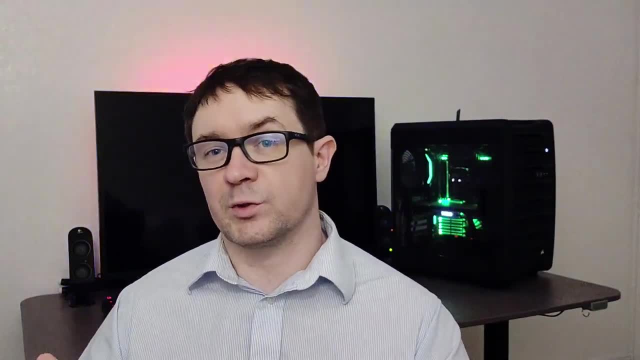 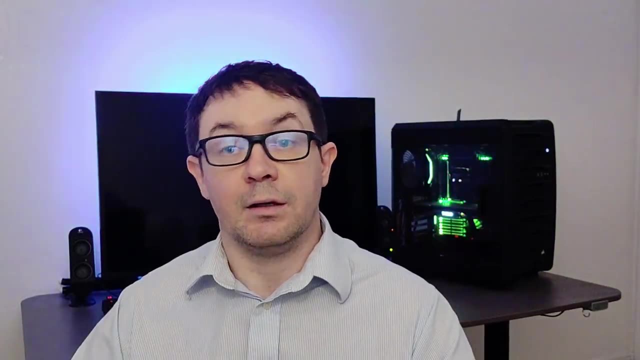 This has the additional benefit that if we don't use a replay buffer, we don't have to store a million transitions, which for trivial environments really doesn't matter. but if you're dealing with something like, say, the Atari library, a million transitions can take up a significant amount of RAM, which can be a limiting factor for enthusiasts. 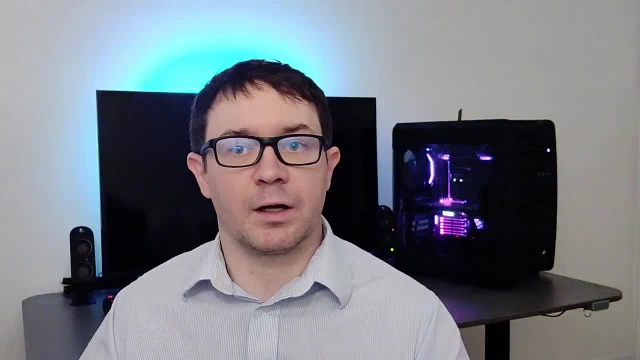 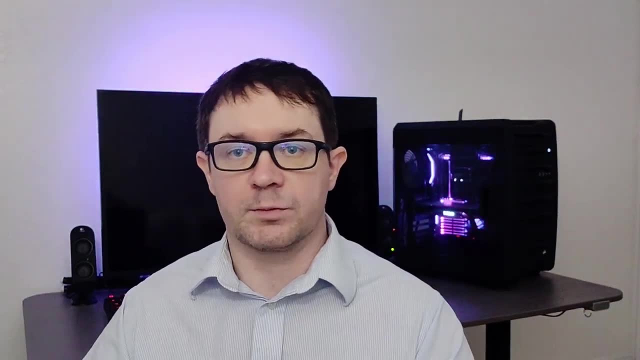 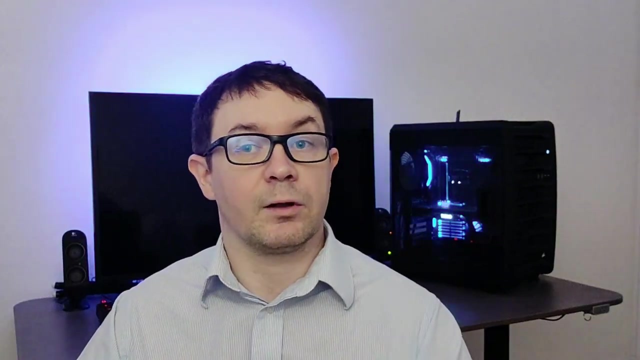 So having the agent play a bunch of different games in parallel on separate environments, only keeping track of a small number of transitions vastly reduces the memory footprint required for deep reinforcement learning. So in what sense exactly is this algorithm asynchronous? What this means exactly in this context is that we're going to have a large number of parallel CPU threads with agents playing in their own environments. 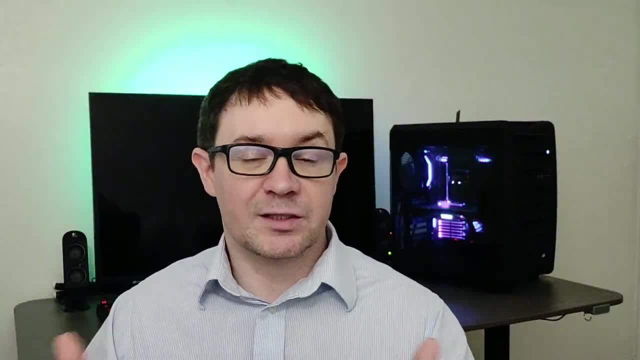 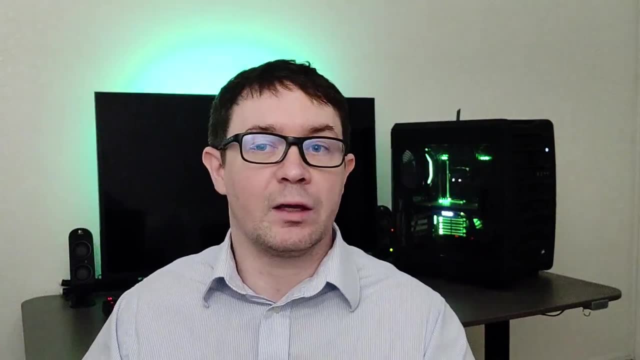 They're going to be acting at the same time, but at various times they're going to be deciding what to do, as well as updating their deep neural network parameters, And so we're not going to have any one agent sitting around waiting on another agent to finish playing the game to update its own set of deep neural network parameters. 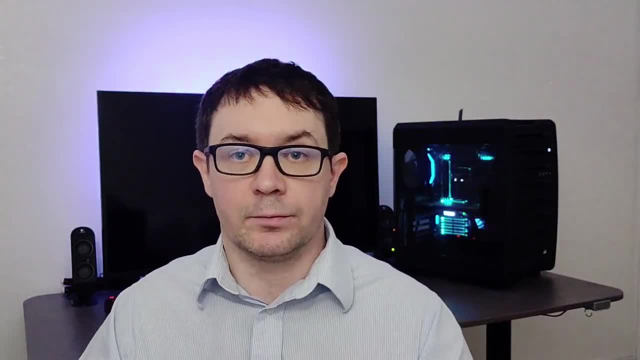 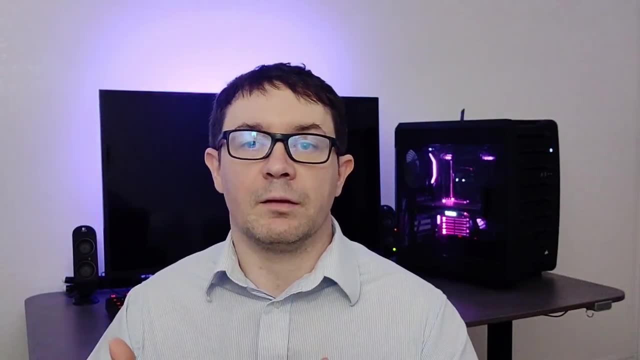 Each one will be totally independent and learning on its own. Now we're not going to be simply throwing away the learning from each agent after it finishes the episode. Rather, we're going to be updating the network parameters of some global optimizer as well as some global actor critic agent. 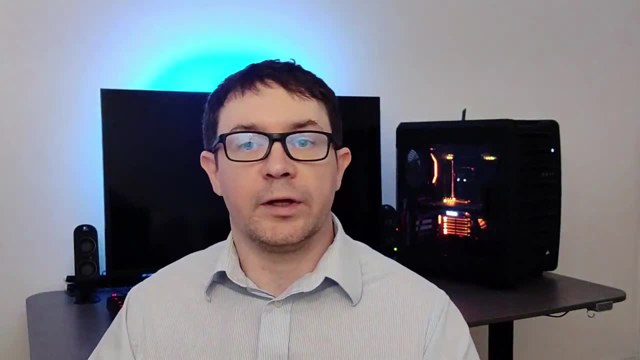 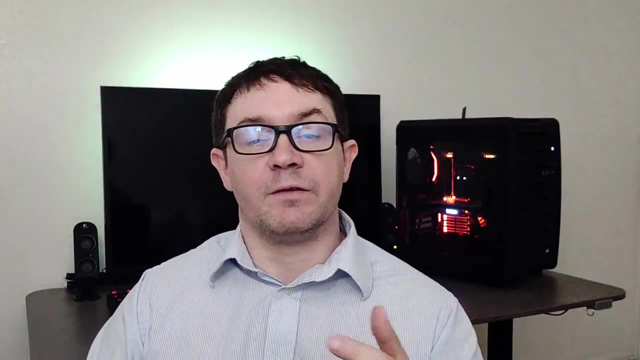 So you have one actor, critic agent that sits atop all of the others and the local agents that do all the learning by interacting with their environments. So what is the advantage? part of A3C. So the advantage essentially means what is the relative advantage of one state. 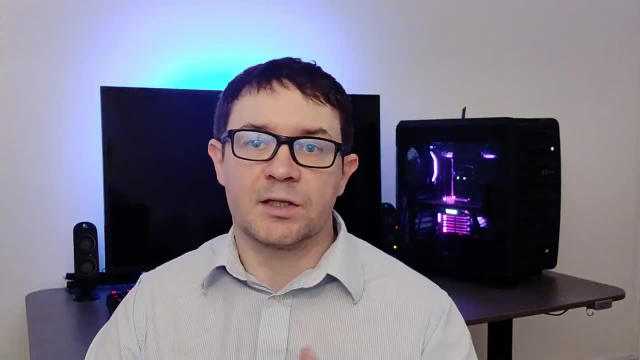 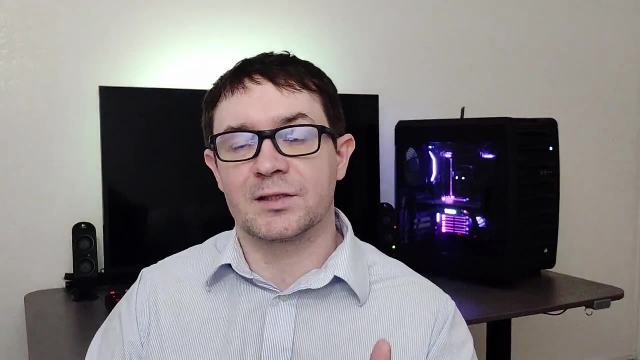 So the advantage essentially means what is the relative advantage of one state. So the advantage essentially means what is the relative advantage of one state over another. It stands to reason that an agent can maximize its total score over time by seeking out those states which are most advantageous or have the highest expected future return. 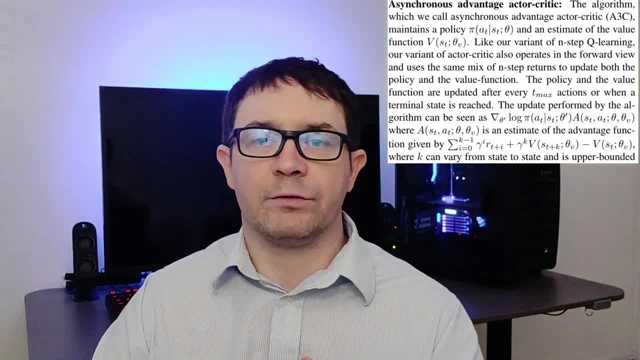 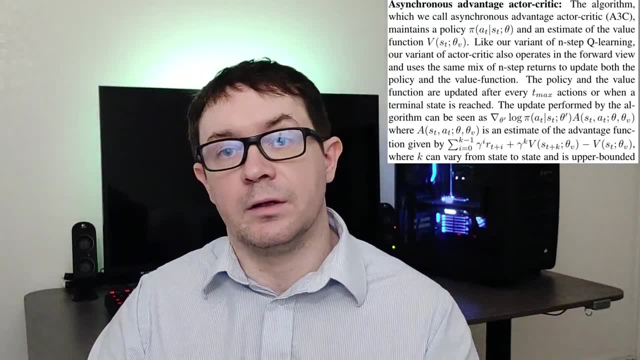 The paper gives a relatively straightforward calculation for this. All we have to do is take the discounted sum of the rewards received over some fixed length trajectory and then add on an appropriately discounted value estimate for the final state the agent saw in that trajectory. Please note that this could be some fixed number, like, say, five steps. 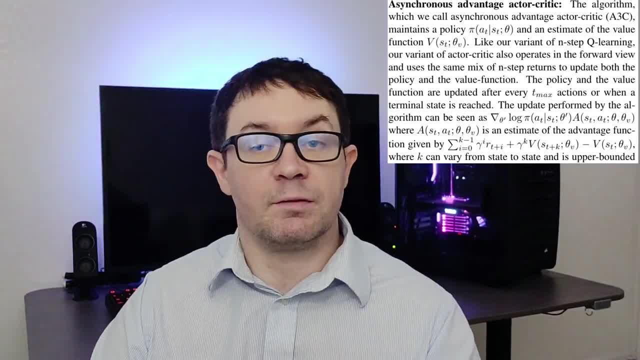 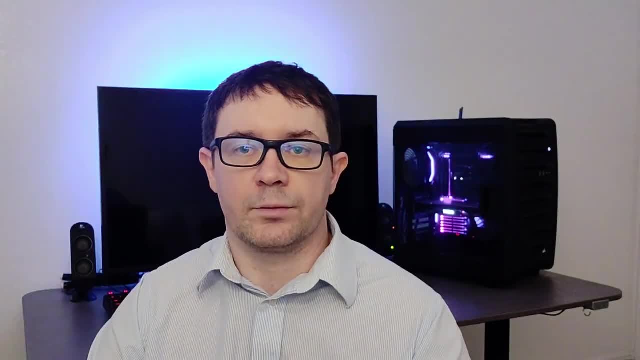 So that way we're always taking the value of the next state minus the current state. So that way we're always taking the value of the next state minus the current state. That's what gives us the relative advantage. That's what gives us the relative advantage. 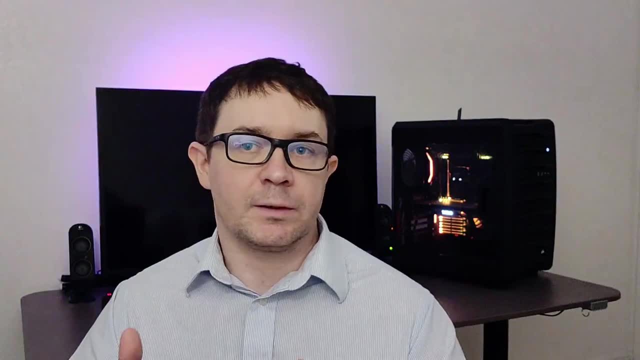 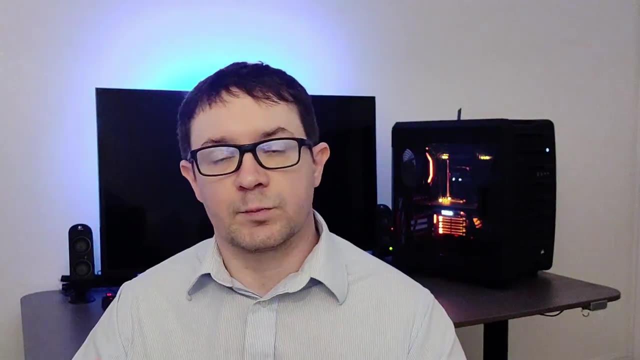 So what does the act-or-critic portion of A3C mean Specifically? this refers to a class of algorithms that use two separate neural networks to do two separate things. So the act-or-network is responsible for telling the agent how to act. Kind of a clever name, right? 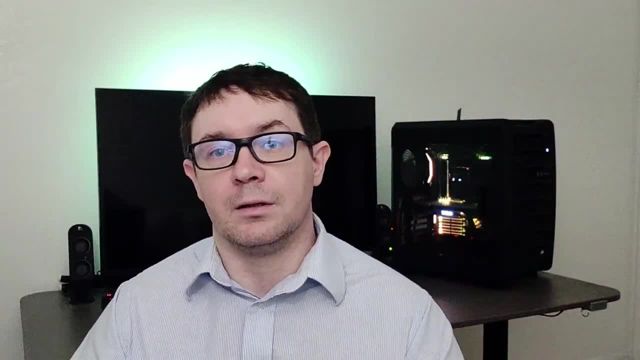 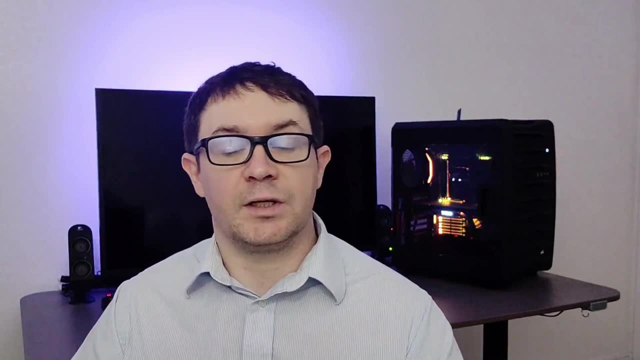 It does this by approximating a mathematical function known as the policy. The policy is just the probability of selecting any of the available actions for the agent, given it's in some state, And so for a discrete action space it's going to be a relative probability of selecting. 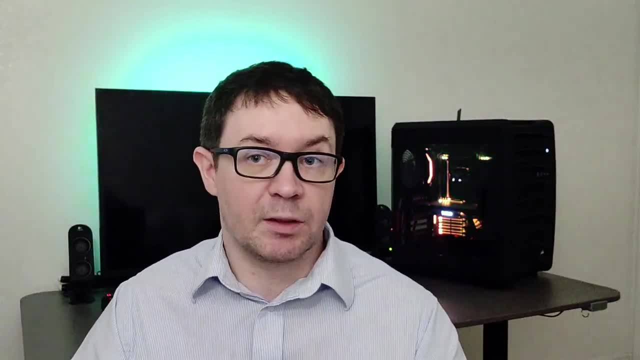 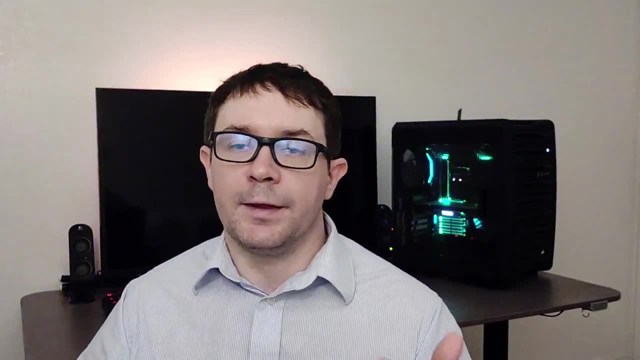 one action over another. So in our cart pull it's going to be, say, 60% move left, 40% move right, so on and so forth. We're going to facilitate this by having two separate networks. The actor network will take a state or set of states as input and output a softmax probability distribution. 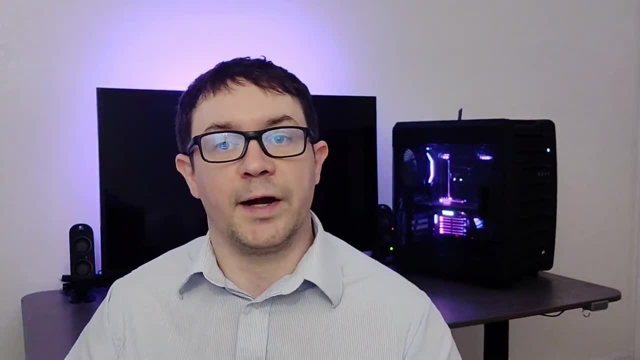 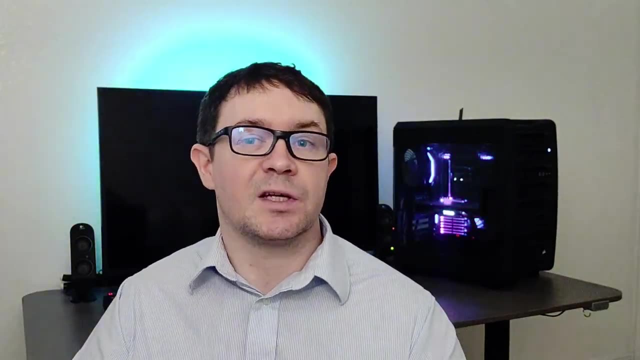 that we're going to be feeding into a categorical distribution from the PyTorch framework. We can then sample that categorical distribution to get the actual action for our agent And we can also use that to calculate the log of the probability of selecting that action. 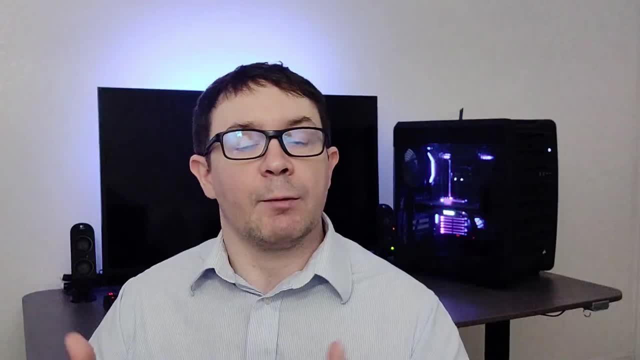 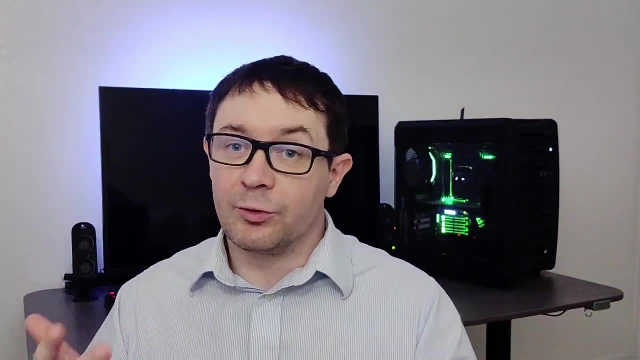 according to the distribution probability distribution and we will use that for the update rule for our actor. Now the critic has a little bit of a different role. The critic essentially criticizes what the agent, the actor, did. It said: you know that action you took gave us a pretty lousy state. 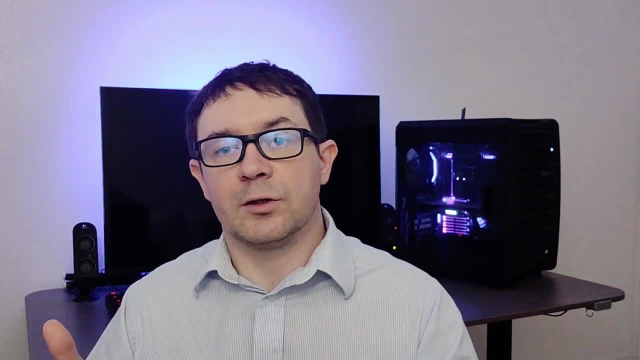 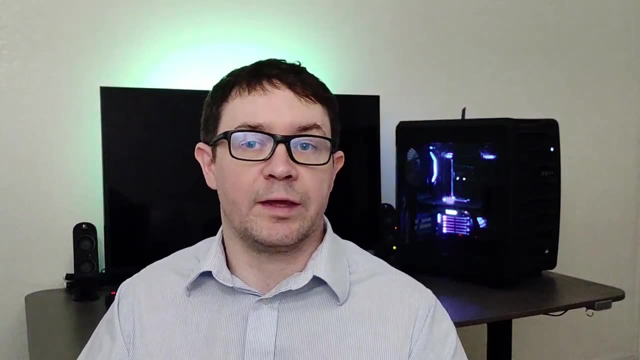 that doesn't have a very large expected future return and so we shouldn't really try to take that action, given that state, any other time that we encounter it. So the critic essentially criticizes what the actor does and the two kind of play off of each other to access more and more. 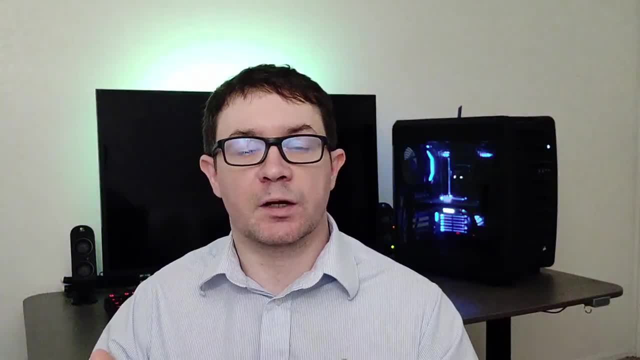 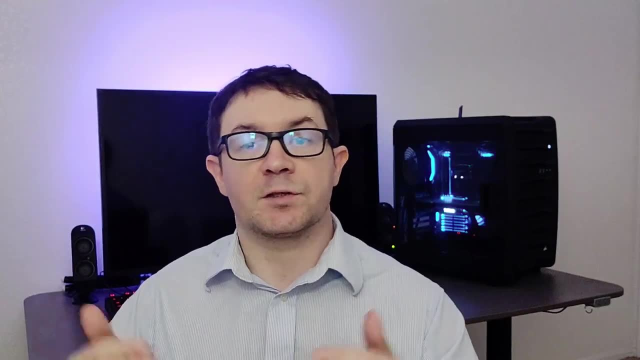 advantageous states over time. Before we go ahead and talk about the specifics of each class, let's get some idea of the general structure and flow of the program. The basic idea is that we're going to have some global optimizer and global actor critic agent that sits on top. 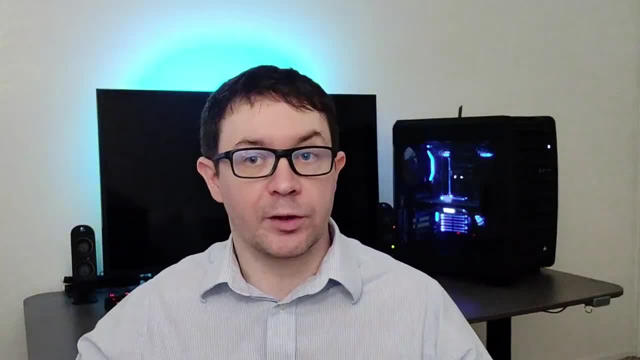 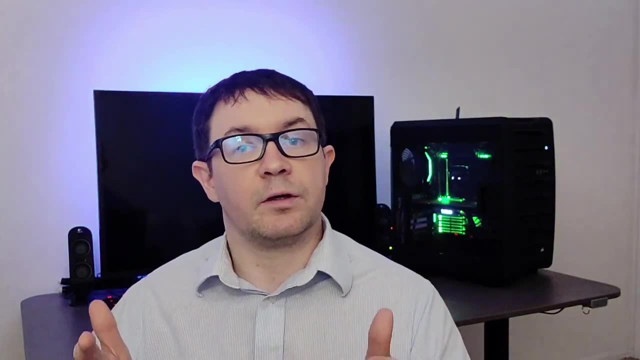 that keeps track of everything the local agents learn in their own individual threads. Each agent will get its own specific thread where it can interact with its own totally distinct and separate environment. The agent will play either some fixed number of time steps or until it encounters a terminal state. 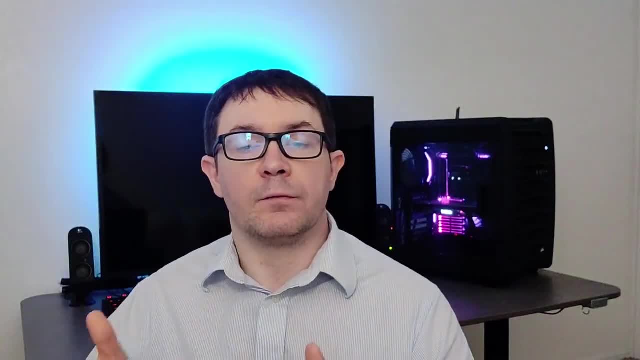 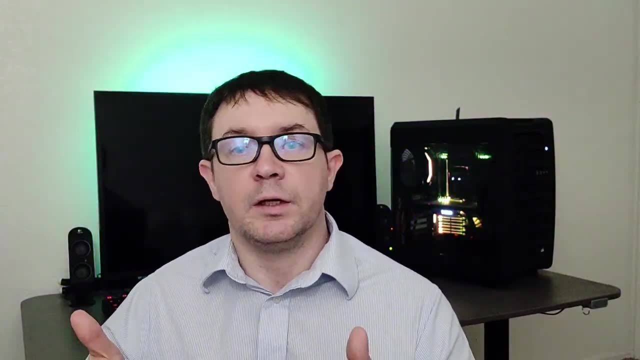 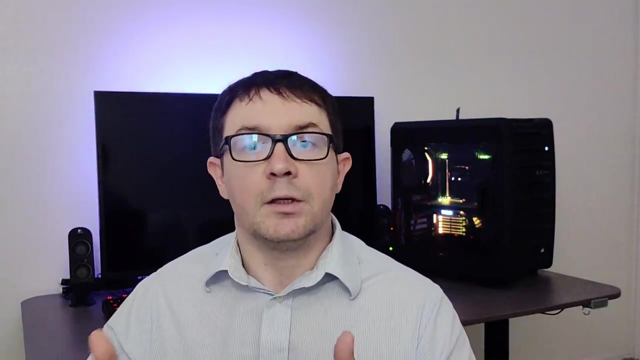 at which point it will perform the loss calculation, to do the gradient descent on the global optimizer. Once it calculates those gradients, it's going to upload it to the global optimizer and then re-download the parameters from that global optimizer. Now, keep in mind each agent is going to be doing this asynchronously. 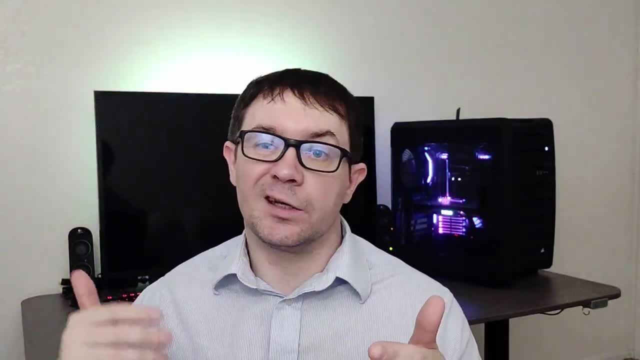 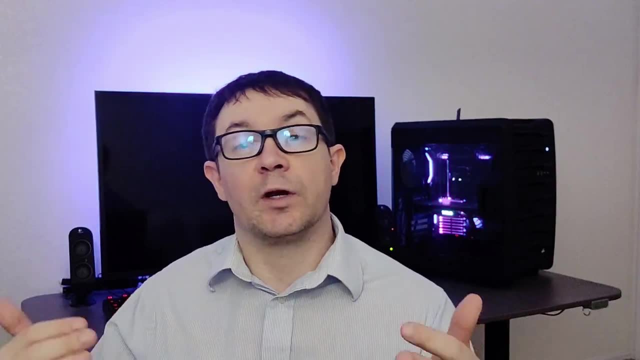 so while one agent is performing its loss calculations, another agent may have already finished that loss calculation and updated the global optimizer. That's why, right after calculating the gradients, we want to go ahead and download the global parameters from the global actor. critic. 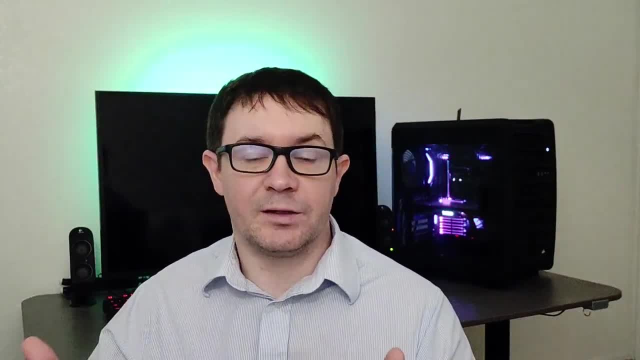 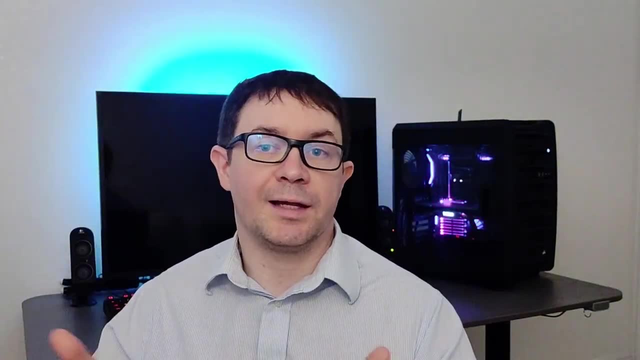 so that way we make sure we are always operating with the most up-to-date parameters. After each time the agent performs an update to its deep neural network, we're going to want to go ahead and zero out its memory so that it can start fresh for another sequence of five. 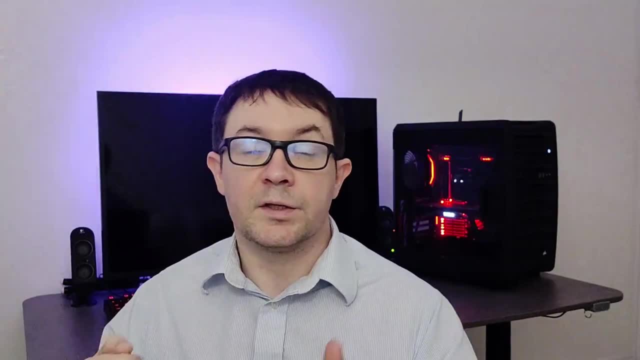 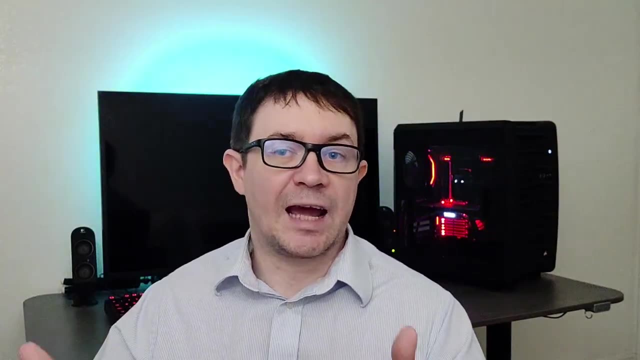 or until it encounters a terminal state number of steps. So now let's talk implementation details. We're going to have a few separate, distinct classes for this, the first of which is going to be overriding the atom optimizer from the base PyTorch package. 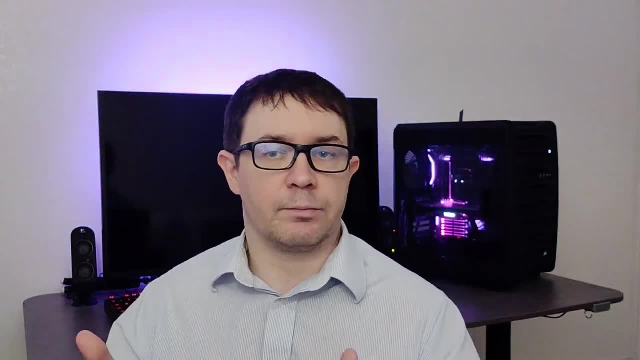 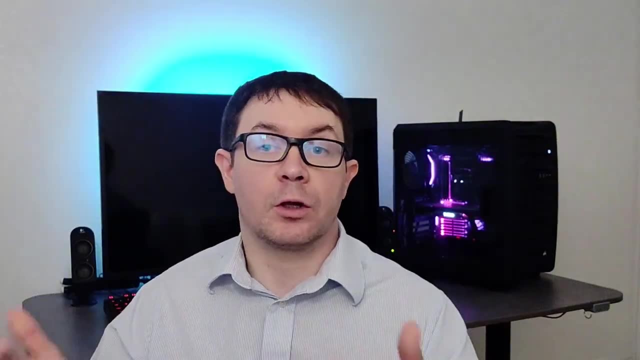 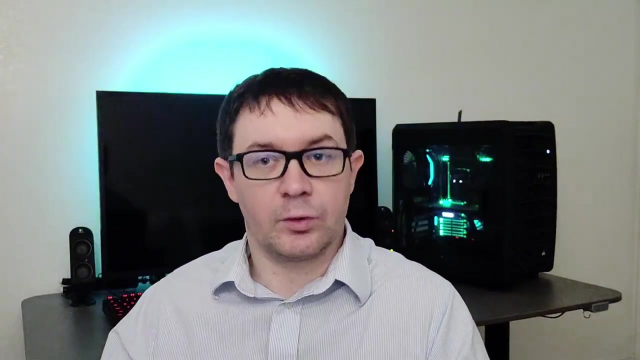 So we're going to have a shared atom class that derives from the base TorchOptimAtom class, and this will have the simple functionality of telling PyTorch that we want to share the parameters of a global optimizer among a pool of threads. It's only going to be a few lines long and it's much easier than it sounds, and I'll show you how to do it in code. 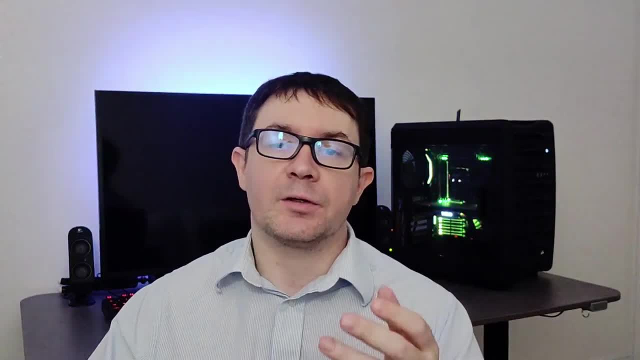 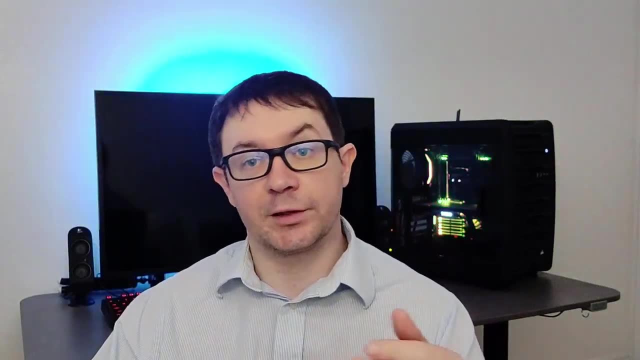 Our next class will be the actor critic network. Now, typically we would use shared input lines, so we're going to have multiple layers between an actor and a critic where we simply have one input layer and two outputs corresponding to the probability distribution Pi and the value network V. 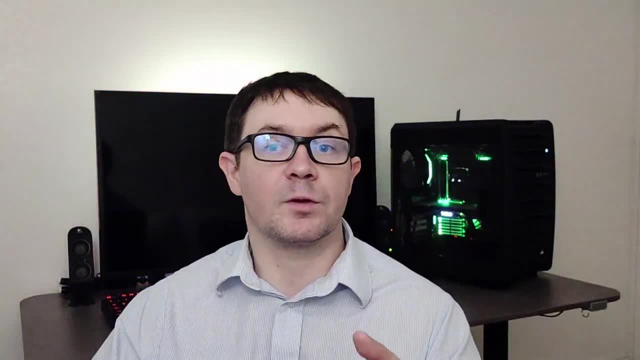 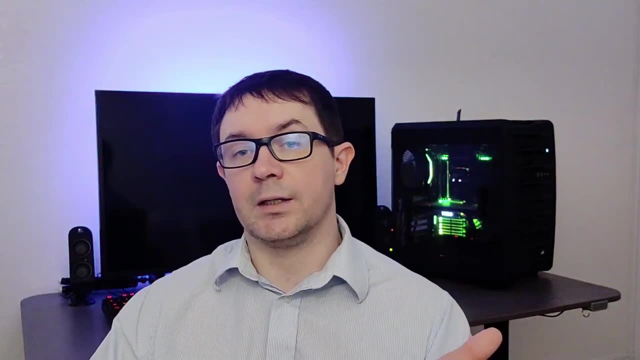 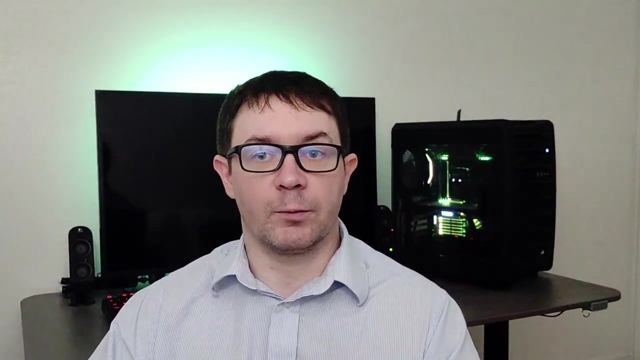 But in this case we're going to host two totally separate, distinct networks within one class. It's a relatively simple problem- the carpool- and so we're going to be able to get away with this. The reason I'm doing it this way is because I, frankly, could not get shared input layers to work with the PyTorch multiprocessing framework. 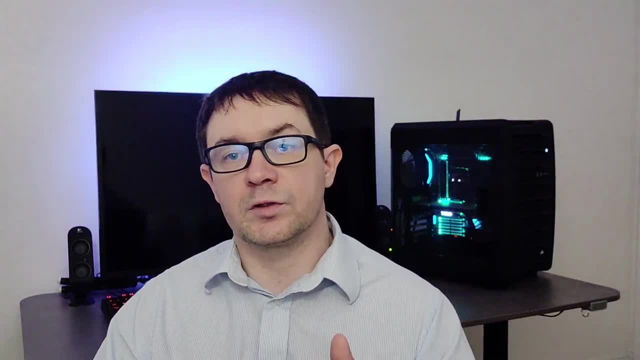 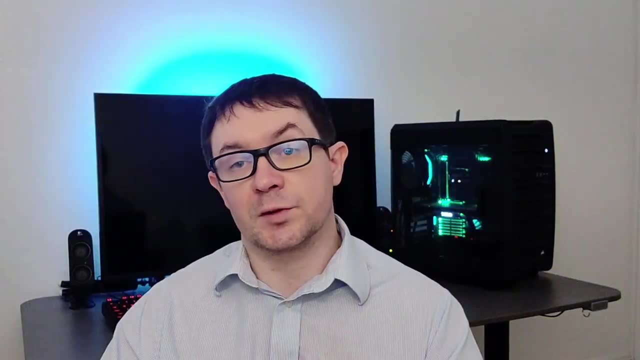 Our agent will also have a memory which we're just going to use simple lists for that. We're going to append states, actions and rewards to those lists and then go ahead and set those lists back to empty lists when we need to clear the agent's memory. 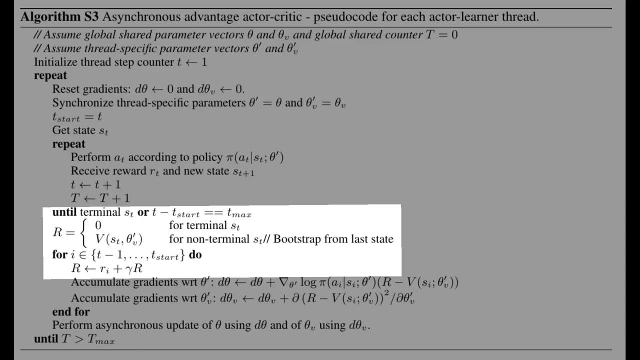 We're going to have a function for calculating the returns, where we're going to use the calculation according to the algorithm presented within the paper. So the idea is that we're going to start at the terminal step or the final step in the trajectory. If that step is terminal, the R or the return gets set to zero. If it's not, it gets set to. 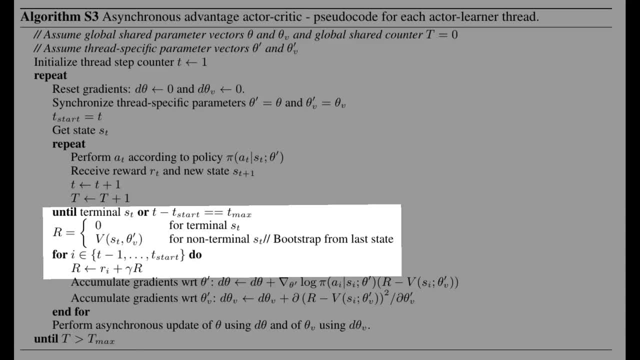 the current estimate of the value of that particular state. Then we're going to work backward from the T minus 1 time step all the way to the beginning and we're going to update R as R sub i plus gamma times the previous value of R. 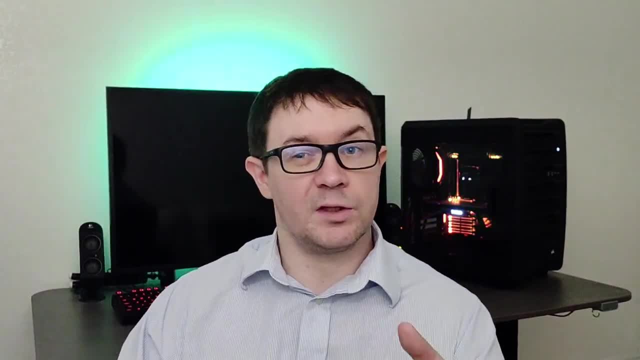 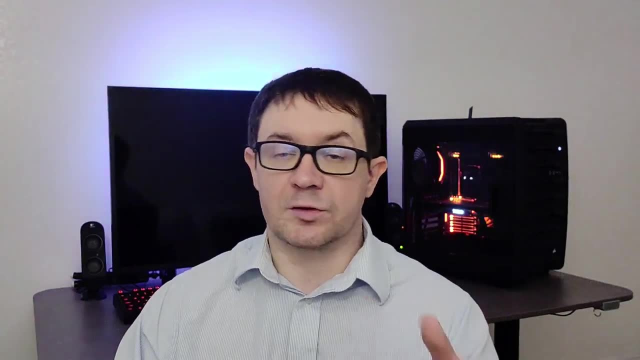 Now I'm going to do a calculation in the video of the coding portion to show you that these two are equivalent, meaning this calculation as well as the earlier advantage description I gave you. I'm going to make sure that you understand that those are actually equivalent and it's just a few lines of mathematics. 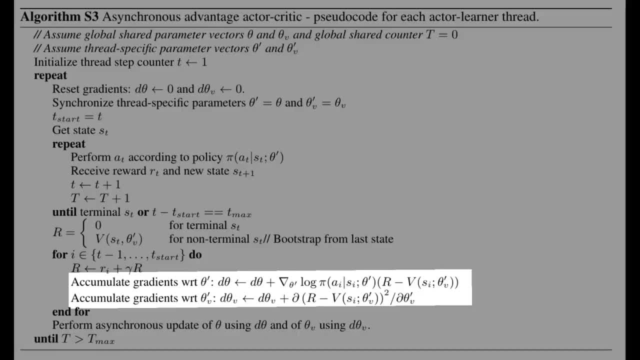 so it's not really that difficult and I've taken the liberty of doing it for you. Then we're going to be calculating the loss functions and these will be done according to the loss functions given in the paper. So for our critic, we're going to be taking the delta between those returns and the values and taking the mean squared error. 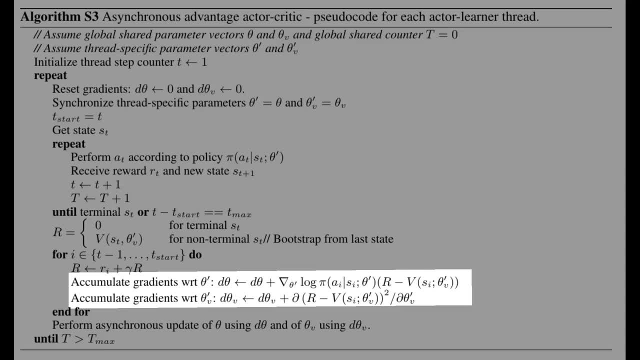 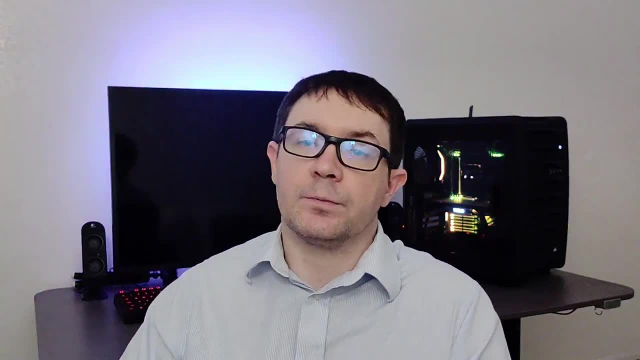 For our actor. we're going to be taking the log prob of the policy and multiplying it by the advantage, and with a negative one factor thrown in there as well. Now, that's a really cool way of calculating the loss for the actor, because it has a pretty neat property. 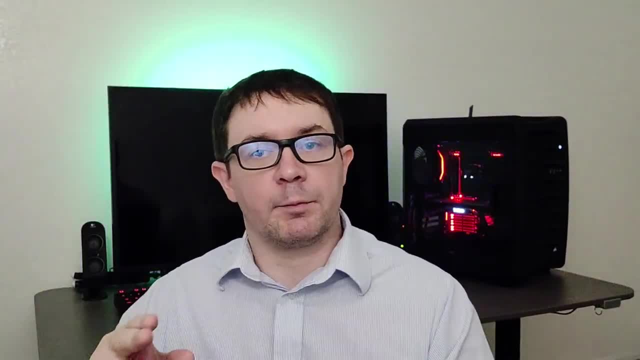 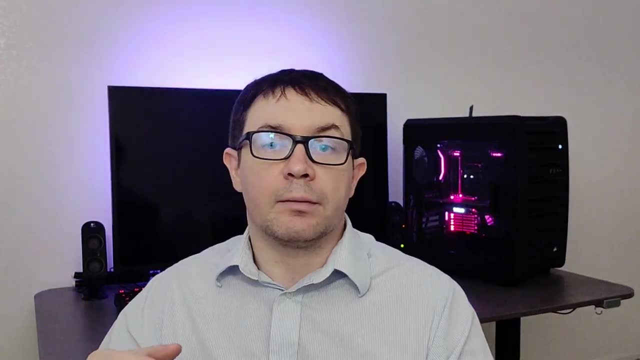 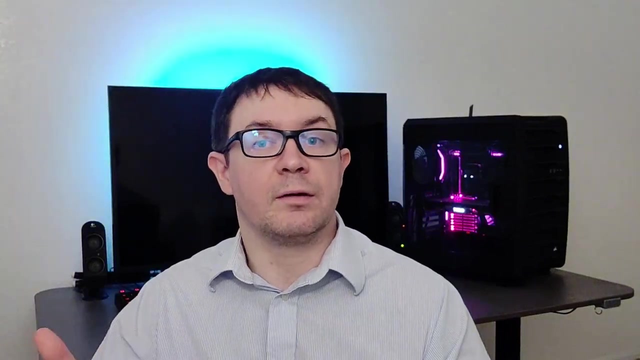 So when we multiply the advantage by the log of the probability, what we're actually doing is weighting probabilities according to the advantage they produce. Actions that produce a high advantage are going to get naturally weighted higher and higher over time, and so we're going to naturally evolve our policy towards being better over time, which is precisely what we want, right. 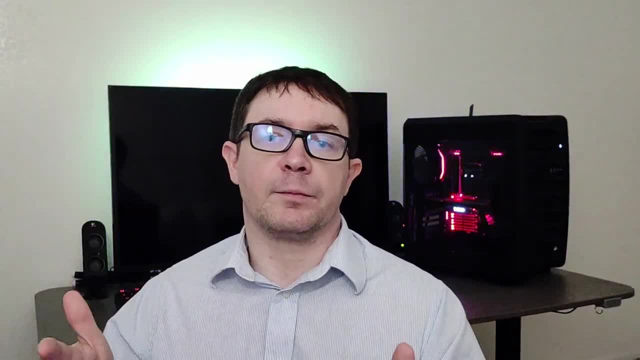 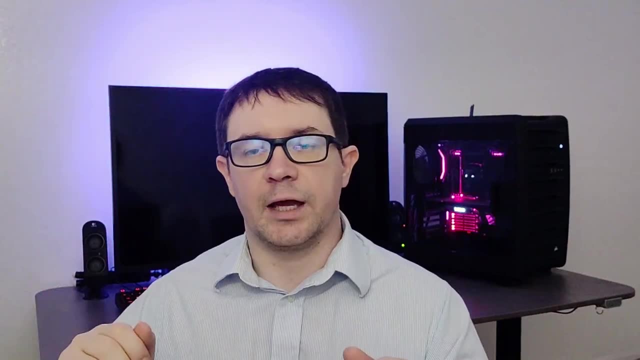 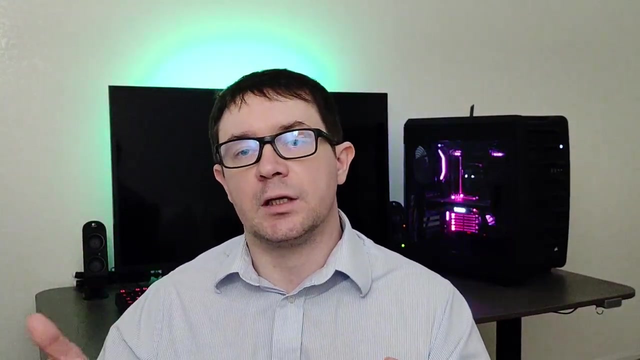 Our final class will be the agent class and this will derive from the multi-processing process subclass. So here's where all of the real main type functionality is going to happen. So we're to be passing in our global optimizer as well as our global actor critic agent, instantiating 16 in. 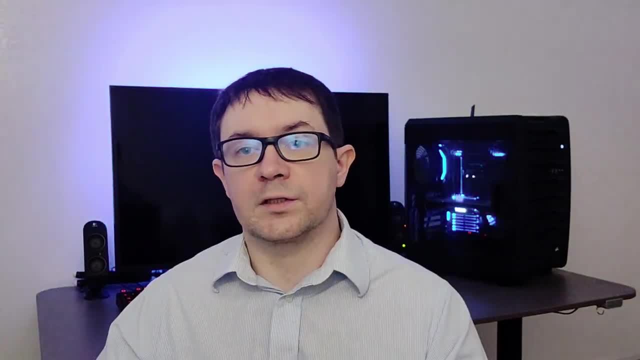 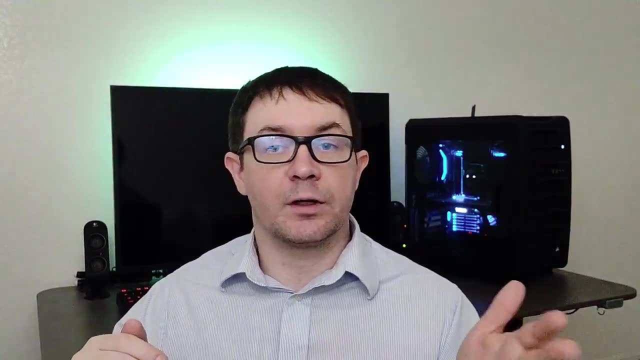 the case of 16 threads for a cpu- local critics- with 16 separate environments, and then each one of those is going to have, you know, two separate loops where it's going to go up until the number of episodes that we dictate and it's going to play each episode as i described earlier within. 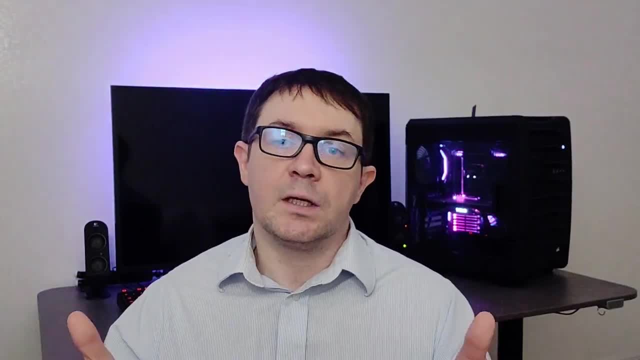 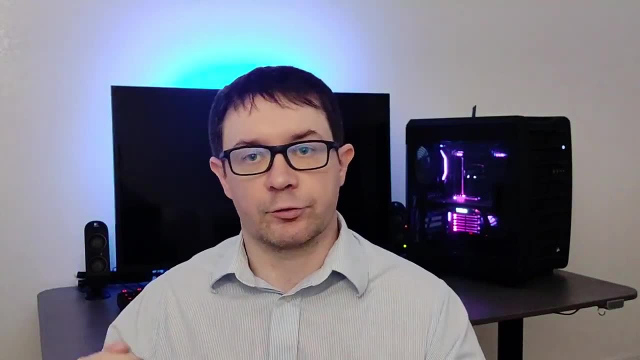 each episode. it's going to play some fixed sequence number of steps and then it is going to perform some update to the global optimizer and then download the parameters from the global actor critic agent. our main loop is basically going to set everything up. we're going to go ahead. 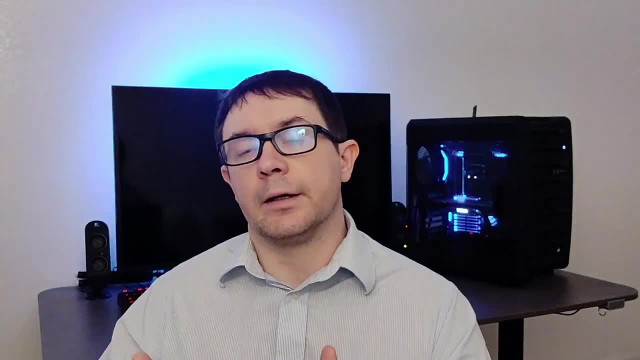 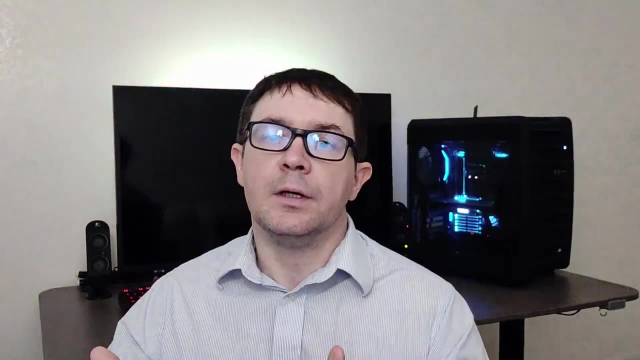 and define all of our parameters, create our global actor critic, our global optimizer, and tell pytorch that we want to share the memory for our global actor critic agent. and then we're going to make a list of workers or agents and then we're going to go ahead and send each of those a start. 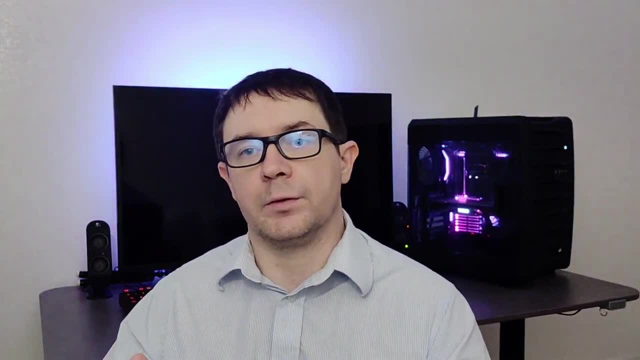 command as well as a join command, so that we can get everything right. and then we can go ahead and balance this out so that we can see if we can determine if that setting, that um for the dual performed view, what it points out, that we can boot difficult load. 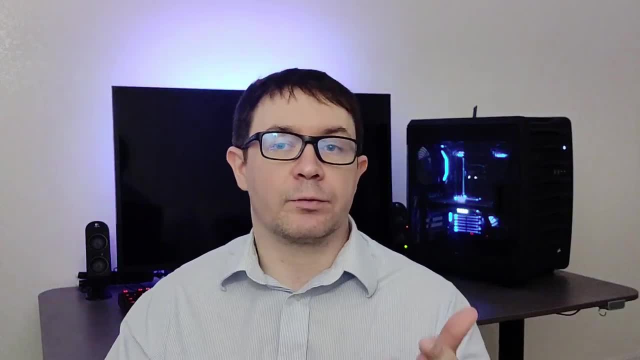 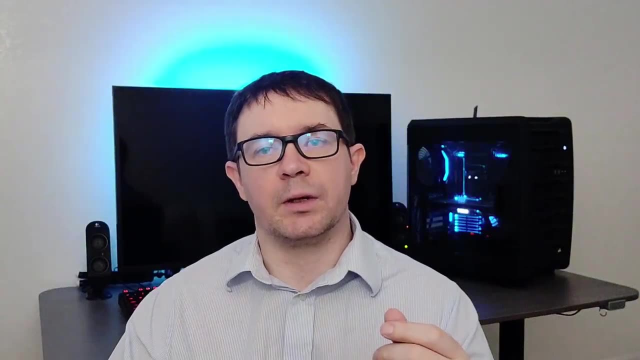 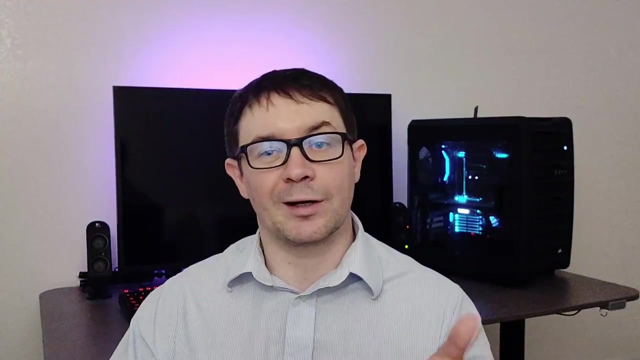 all right, so that's another additional video, but that's basically all that we have for this one. so let's try out the control video here. here's what it looks like while we're in the radio. so that's the same way. i literally already, honestly, i. 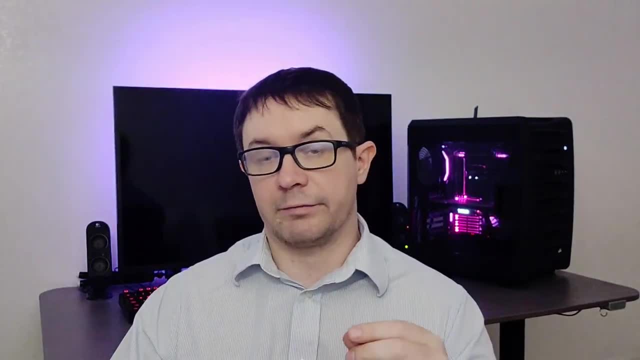 don't remember the software going out, but the lateral rendition of the Lazure workstation doesn't have this echelon anything to, can you? So what are some critiques of this algorithm overall? well, one is that it is exceptionally brittle, so it's highly sensitive to initial parameters. you can solve this by setting global seeds for 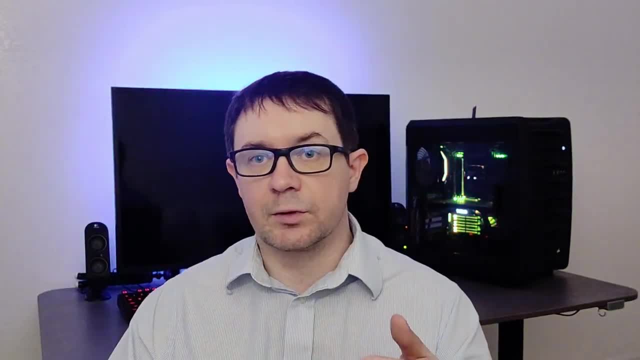 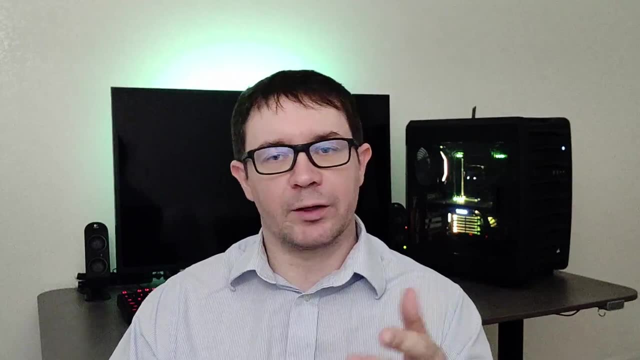 the random number generators so that you're getting consistent random numbers over time and so you're going to know exactly how you're starting. but to me it's a little bit kind of like cheating, so i don't do it in this video, but it is something to take note of and in the original 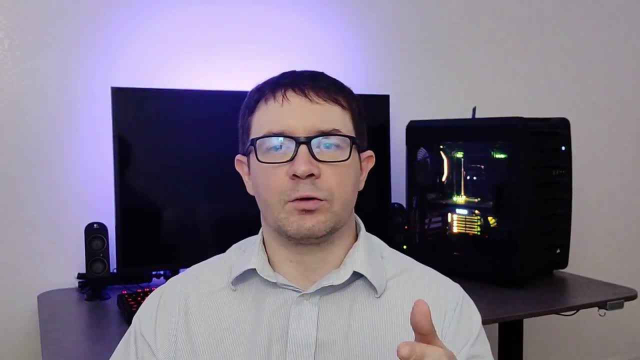 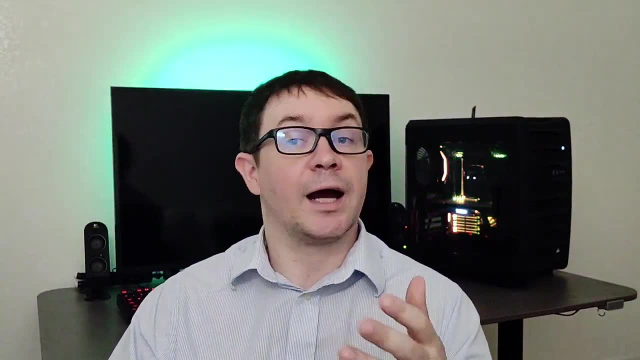 paper. i think they do something like 50 different runs of each evaluation, some large number to get a pretty tight or to get a pretty solid distribution of scores, and that is, i think, because of the high degree of run to run variation. okay, i have lectured at you enough again, if you like. 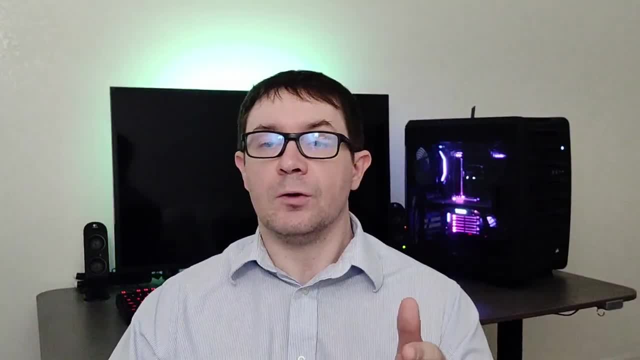 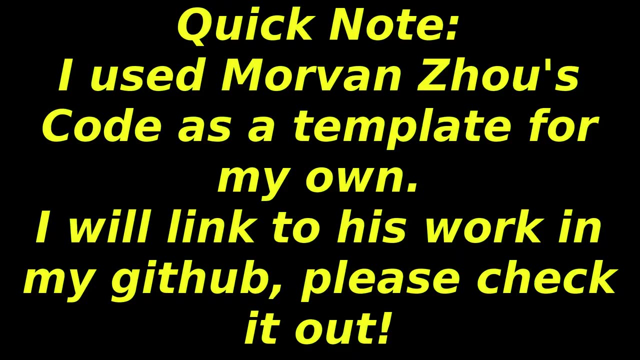 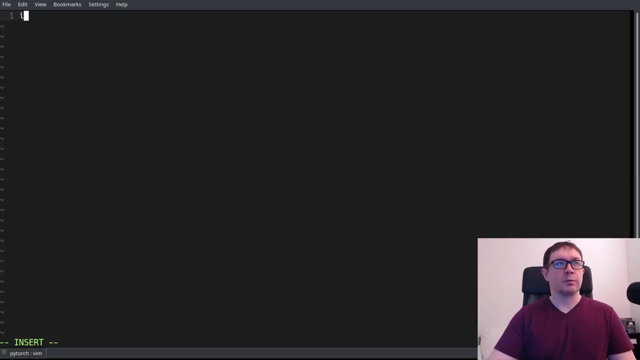 to read written content. i have a link in the description to a blog post where i talk about this in a little bit more detail, but nonetheless, let's go ahead and jump right into the coding tutorial. let's go ahead and start with our imports. let's go ahead and start with our imports. 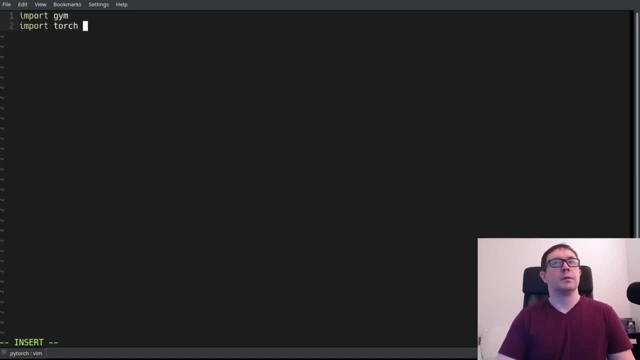 we will need jim for our environment. we'll need our base torch package. we'll need torch multi-processing to handle all the multi-processing type stuff. we will need torch nn to handle our layers. we'll need nn functional to handle our activation functions and we're going to need our distribution as well. 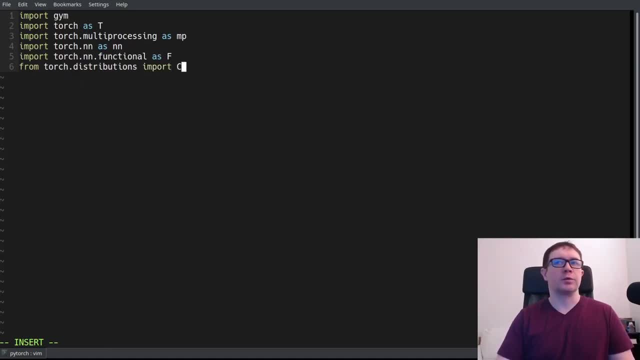 and in this case we're going to need a categorical distribution. all this does is takes a probability output from a deep neural network, maps it to a distribution so that you can do some actual sampling to get the real actions for your agent. now i want to start with the shared atom class. this will handle the fact that we are going to 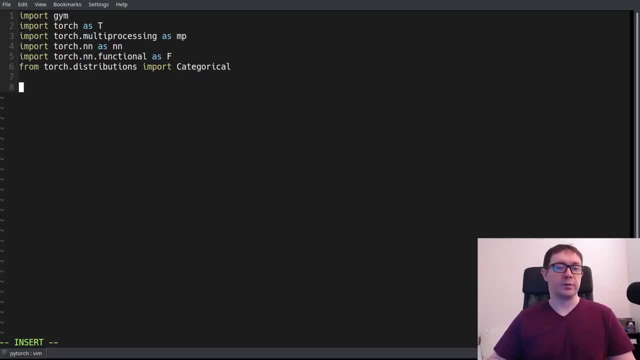 be sharing a single optimizer among all of our different agents that interact with separate environments. all we're going to do here is call the base atom initializer and we're going to call the base atom initializer and then iterate over the parameters in our parameter groups, setting these steps exponential average and exponential average squared to zeros effectively, and then 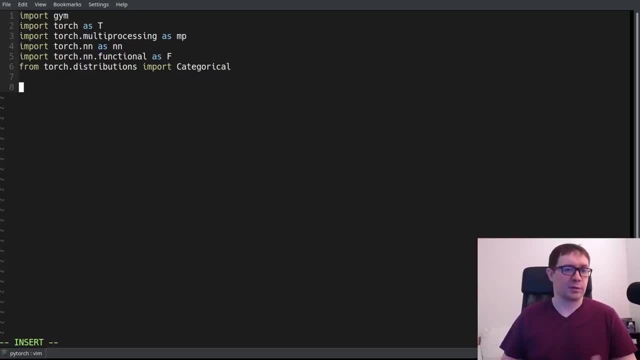 telling it to share those parameters amongst the different pools in our multi-threading pool, and this will derive from the base atom class. our default values are going to be, i believe, identical to the defaults for the atom class, and then we want to call our super constructor. 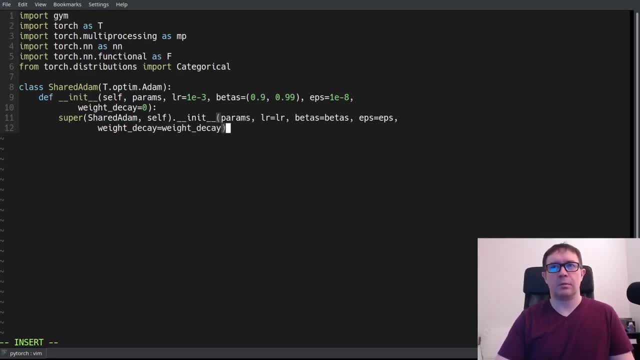 now we're going to handle setting our initial values and then we're going to tell torch that we want to share the memory, for our parameters are for our gradient descent and note the presence of the underscore at the end of memory there. okay, that is it for the shared atom. pretty straightforward. 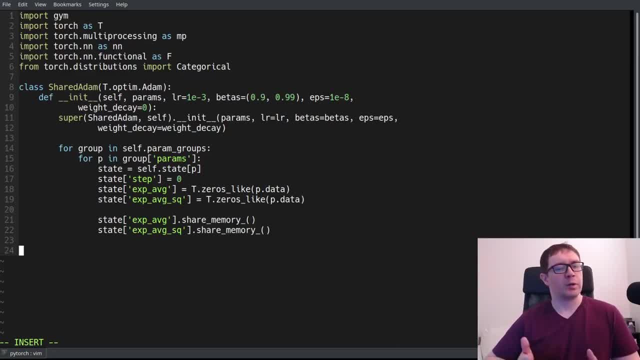 next up we want to handle the actor critic network, which will also encapsulate a lot of the functionality i would typically put into an agent class because of my understanding of the design principles of object oriented software programming. in this case, i have to shimmy a few things around because the agent class is going to handle the 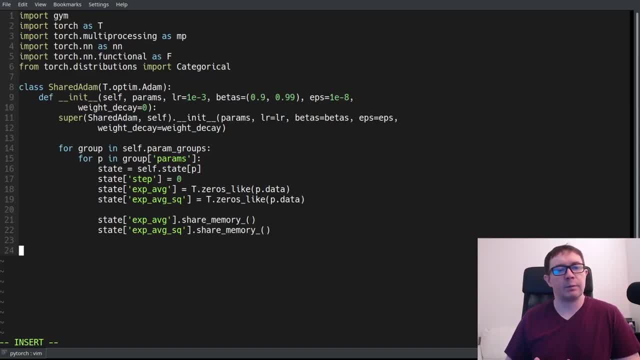 um, multi-processing elements of our problem, and so it doesn't really make sense to stick this uh like the choose action or memory, uh, memory functionality- in the agent class. so we're going to stick it in the network class. it's not a huge deal, it's just a departure. 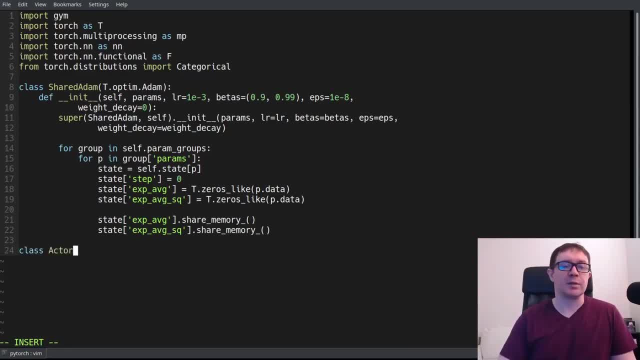 from how i normally do things, and certainly not everybody does things the same way i do. so our initializer takes input dims from our environment. um, we have a number of actions from our agent and a default value for gamma of 0.99. we also have to save our gamma and the next thing we want to handle is writing our actual 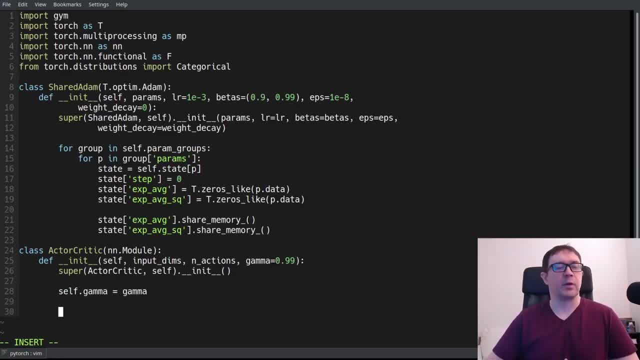 deep neural network. now, this is also a little bit different than the way i normally do things. normally, i would have a shared input layer that branches out into a policy and a value network as two separate outputs with that shared input layer. when i tried to do that, i found that the 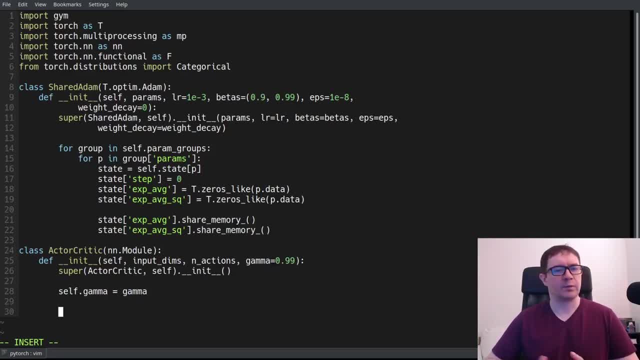 software doesn't actually run. it doesn't handle the threading aspect very well in that case, when you have shared input layers- uh, from a deep neural network. i don't know exactly why that is. if you know, please leave a comment down below, because i'd be very curious to hear the explanation. 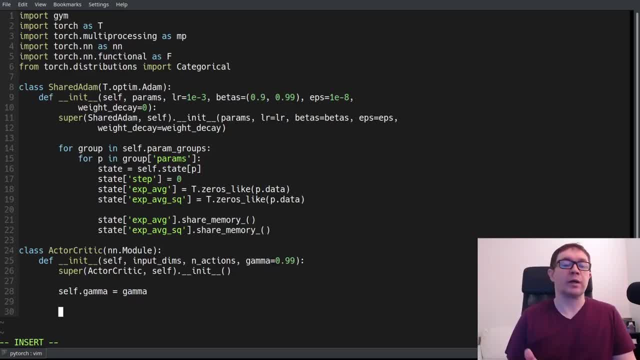 it's simply what i found out through my own experimentation. so we're going to have two separate inputs- one for the policy and one for the value network- as well as two separate outputs, so they're effectively two distinct networks within single class, and we're only going to be using 128 neurons here, not a very large. 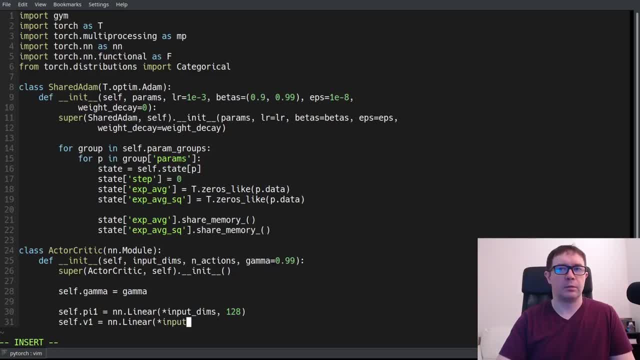 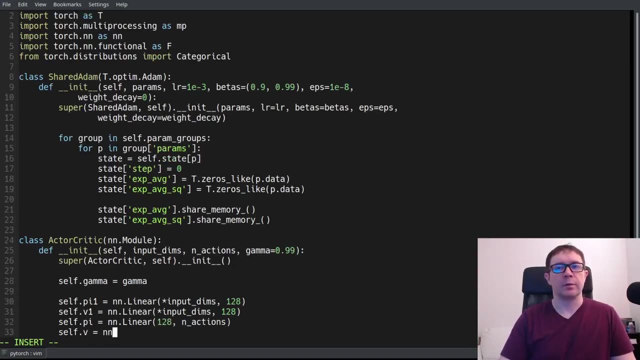 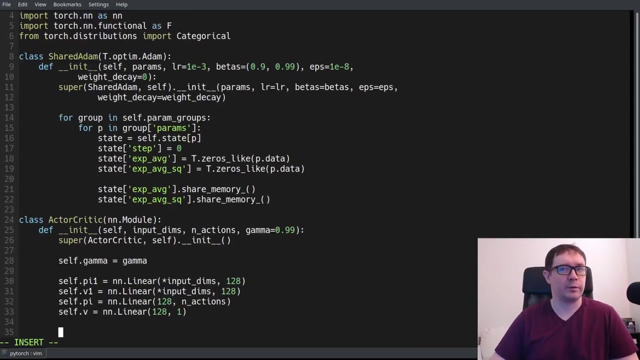 network and our output will take those 128 hidden neurons and convert it into number of actions and our value function will take likewise 128 hidden layers, hidden elements, and convert it to a single value. or if you pass in a batch of states, a batch of values, the agent also- excuse me, the network also has some. 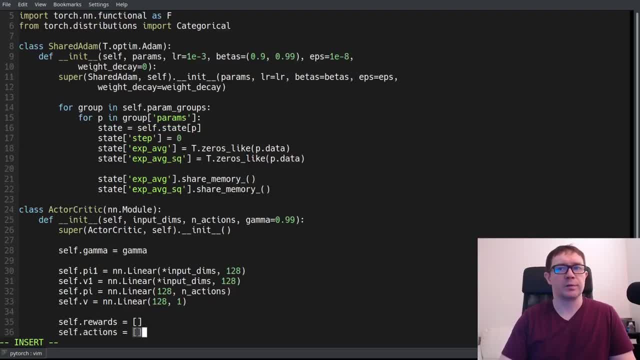 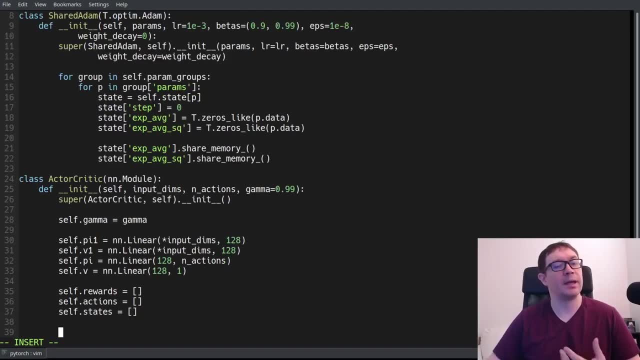 basic memory. so rewards, actions and states. these we will handle just by appending stuff to a list and then, and each time we call the learning function, we're going to want to reset that memory. so let's go ahead and handle that functionality first. so the remember just appends a state action. 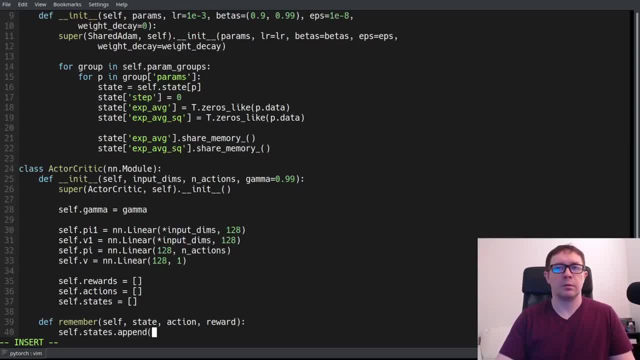 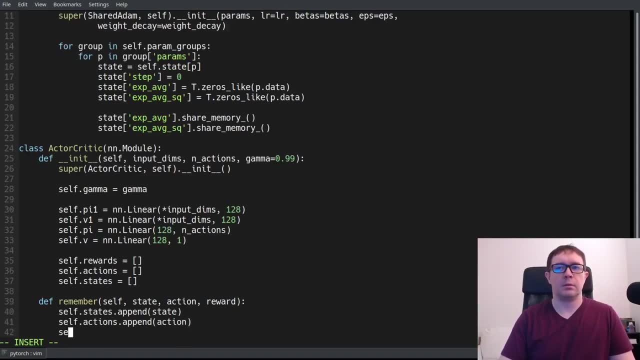 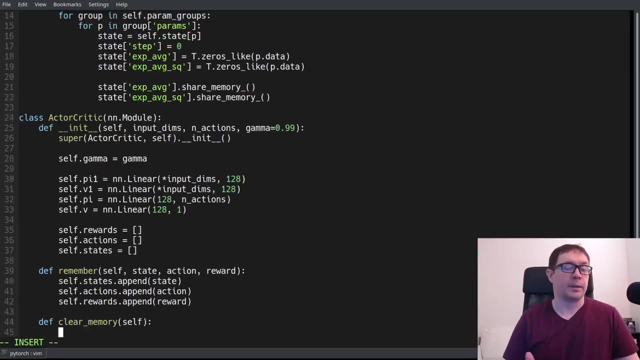 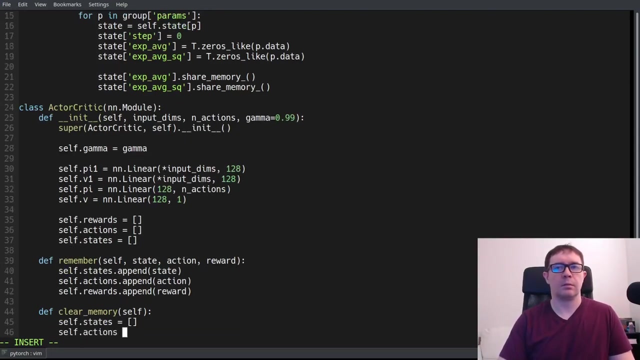 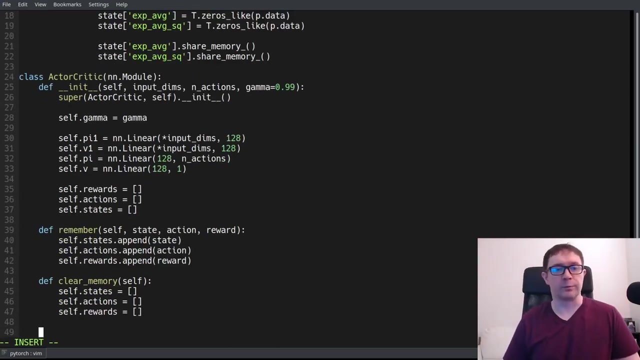 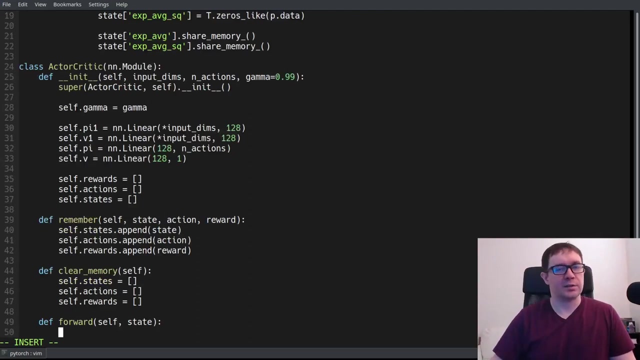 reward to the relevant list and a clear memory function just zeroes out all those lists- pretty straightforward. next we have our feed forward function that takes a state as input. so we're going to pass that state through our first input layer for our policy and perform a relu activation. 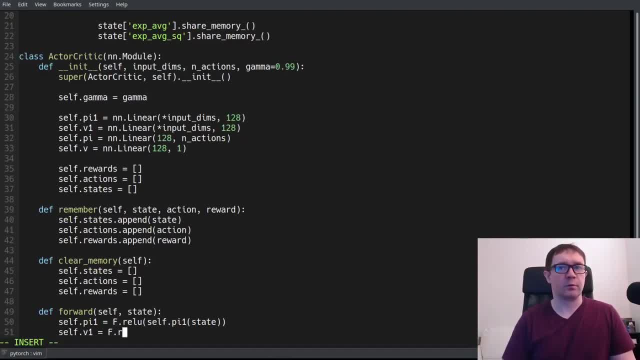 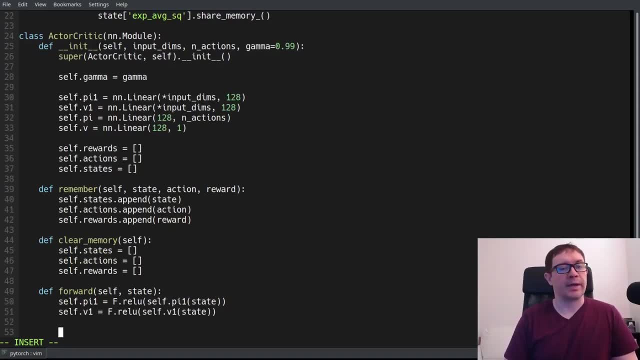 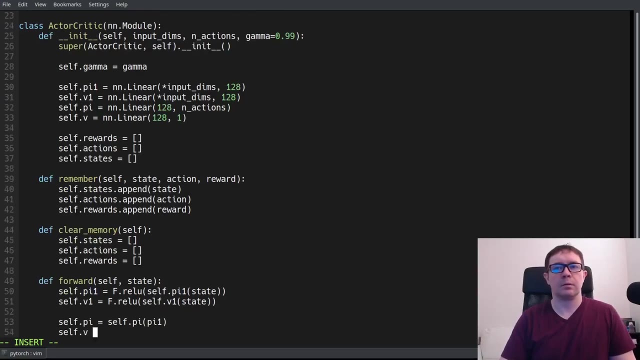 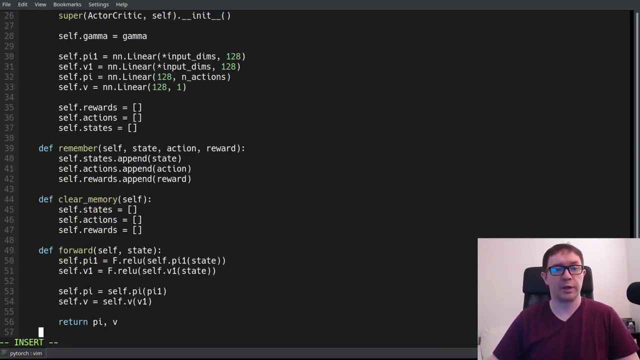 on that and do something similar for the value input layer, and the outputs of those two are going to be passed to the rel, to the relevant policy and value outputs, and then we just return PI and V- pretty straightforward yet again. next we're going to have our function to calculate the returns from our sequence. 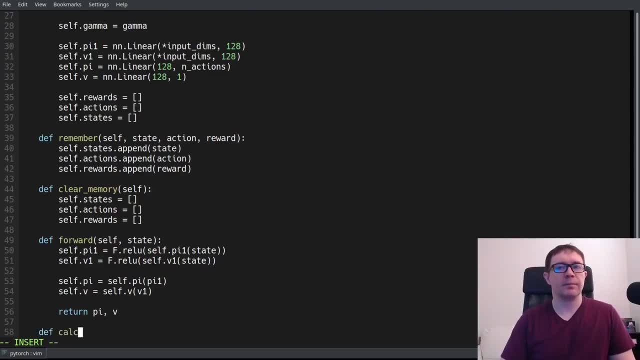 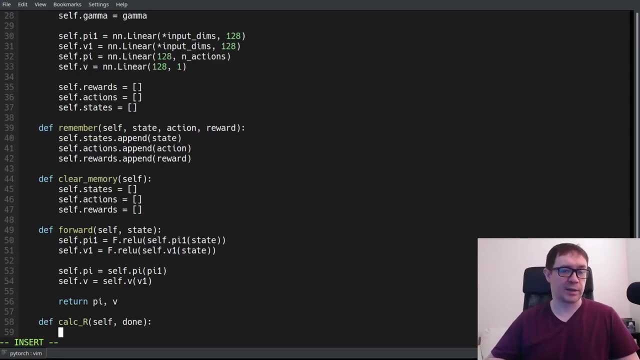 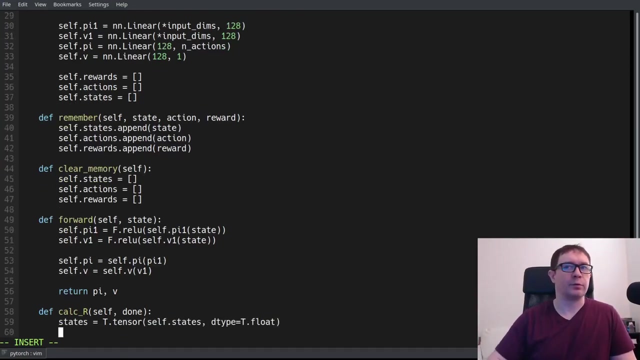 of steps. so this will only take a single input and that will be the terminal flag. recall that the return for the terminal step is identically zero, so we need the terminal flag or the done flag to accommodate that. so we want to go ahead and convert the states from our memory to a torch tensor of tfloat data type, because it is a little. 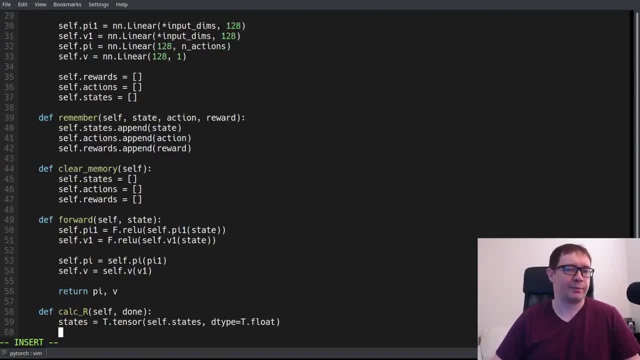 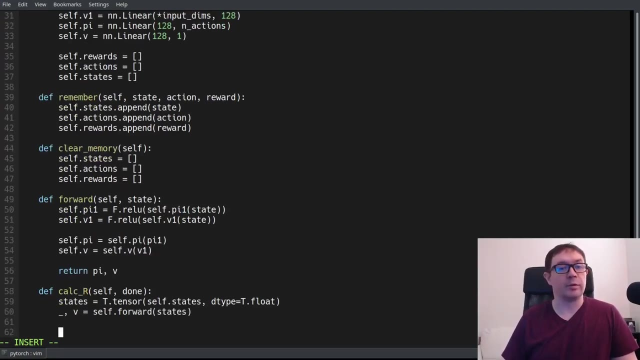 particular about the data type. you don't want to pass it in double. it gives you an error. so you can draw out the advantage here. we're going to limit it, and we're going to limit it by tradingί, agree. and we're going to subtract that by x to Harsh the nouvelle. 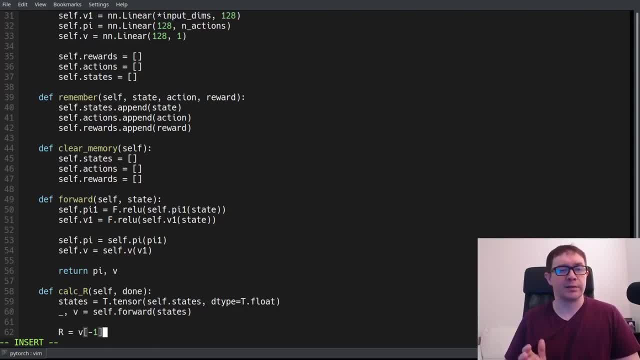 egg of these three states, there are four divider, and f to the positive. so what we want is two foes in the order of x del squared plus x to x to the negative. so we want to be able to atGAN and done so that if the episode is over, one minus done is zero. so you're multiplying by zero. you. 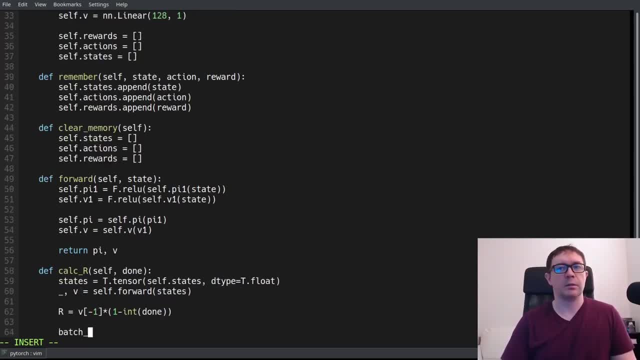 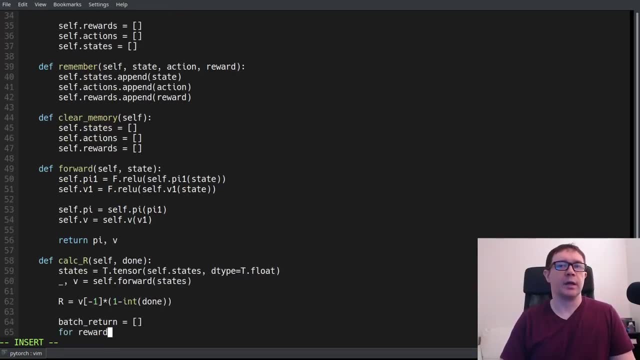 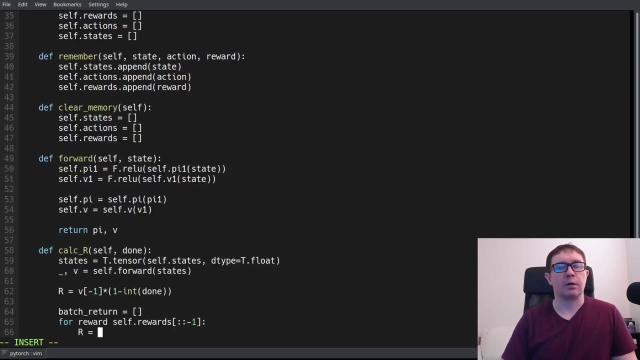 get zero. pretty handy way of handling that. then we're going to handle the calculation of the returns at all the other time steps. so we're going to go ahead and iterate over the reversed memory and say that our return is the reward at that time, step plus gamma, times r, and then just return. 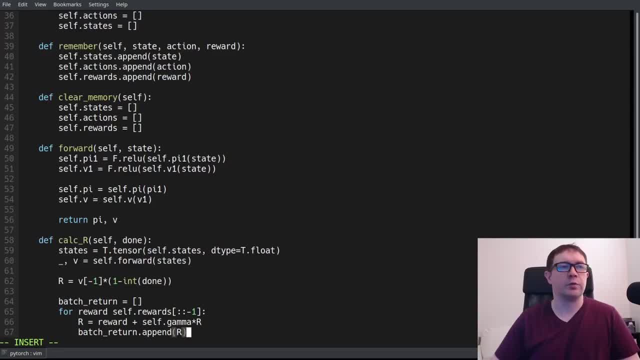 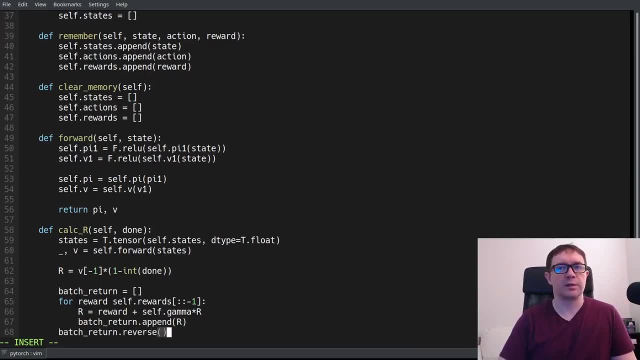 excuse me, append that return to the list of batch returns and then, finally, at the end, you want to go ahead and reverse that list again. so that's in the same order in which you encounter the states. this calculation reverses it because you're starting at the end, when you know the value of. 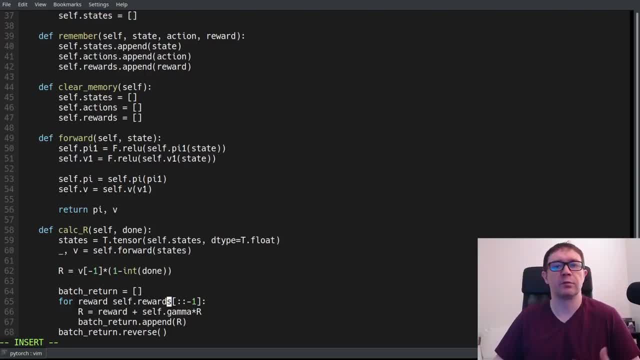 the final state, or at least the estimate of the value of the value of the final state according to the critic, and then reversing it to get it back in order for passing it into our loss calculation function. now, this may be a strange form to you. if you write it out by hand, maybe i 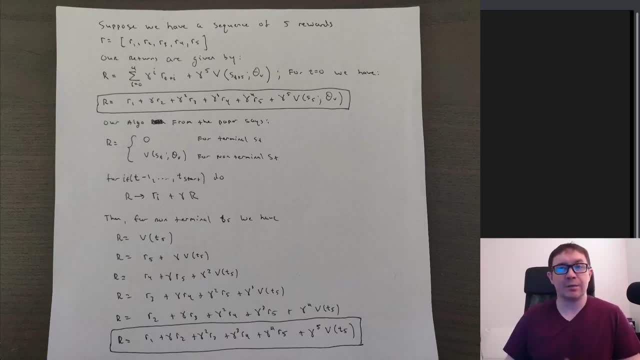 can show you something here where i did it for you. if you write it out by hand, this particular chunk of code, you can see that it's identical to what they tell you. the calculation is in the paper. so, yeah, you can do that exercise on your own to convince yourself, or i can just show it to you. so 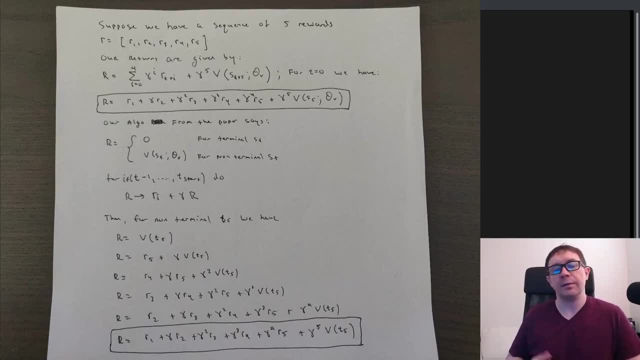 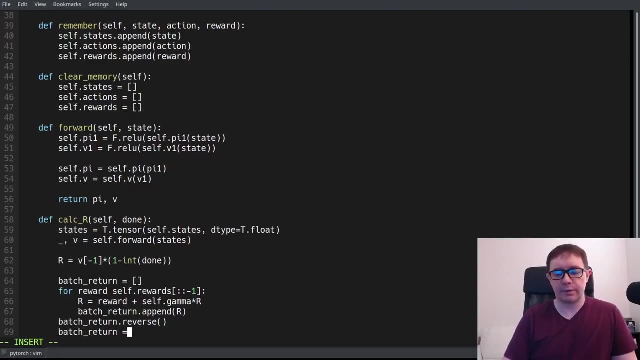 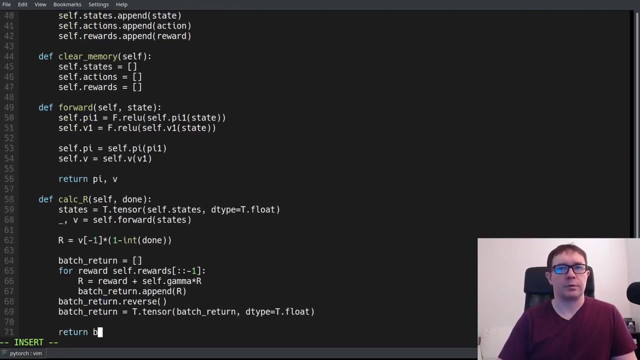 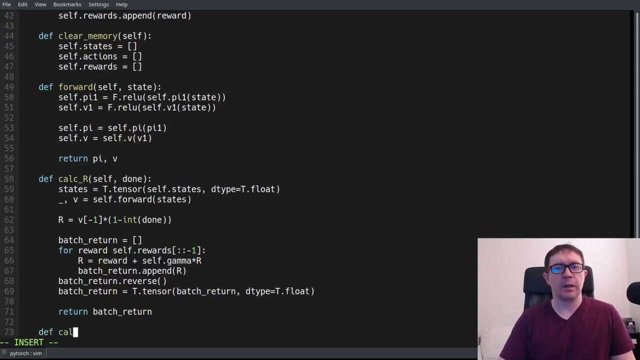 that i can convince you of it, but this is indeed the return calculation from the paper. everything is as it should be, and then i want to convert that to a tensor and return it. next we have to handle the calculation of our loss function, and this again is: 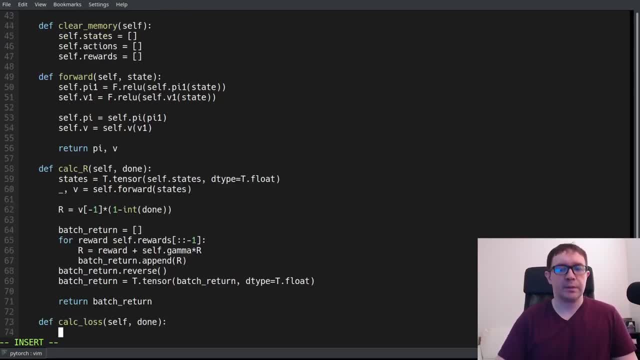 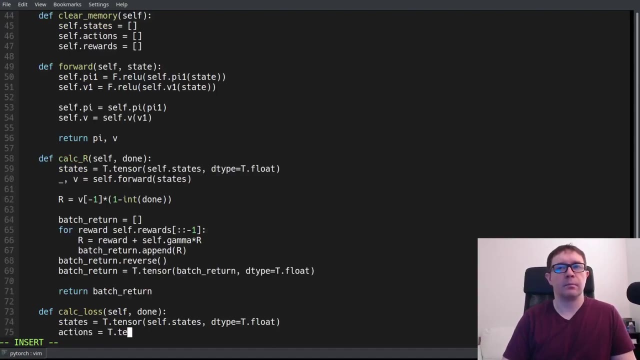 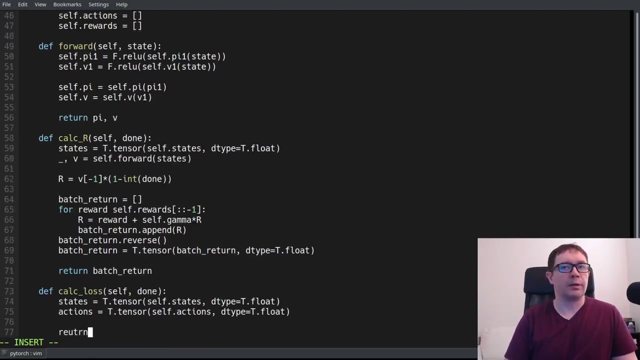 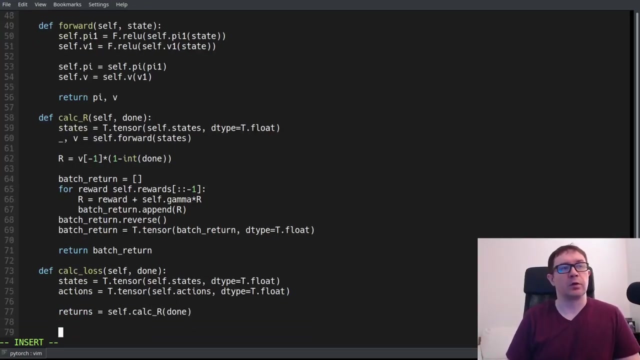 only a single input, the terminal flag from the environment. we're going to go ahead and get the value- excuse me, the tensor representations of our states and actions right at the beginning, and then we're going to go ahead and calculate our returns and then we're going to perform the updates. so we're going to be passing. 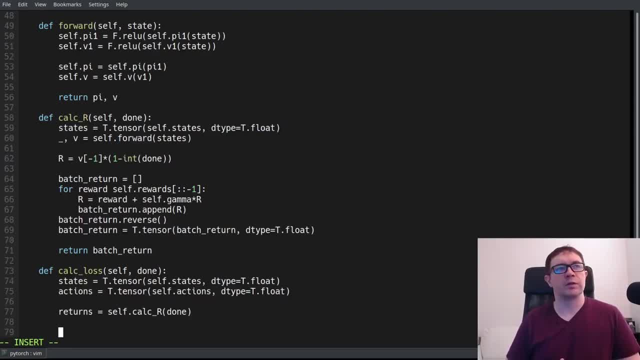 the states through our after critic network to get the new values as well as then a distribution according to the current values of our deep neural network. we're going to use that distribution to get the log probes of the actions the agent actually took at the time. it took them and 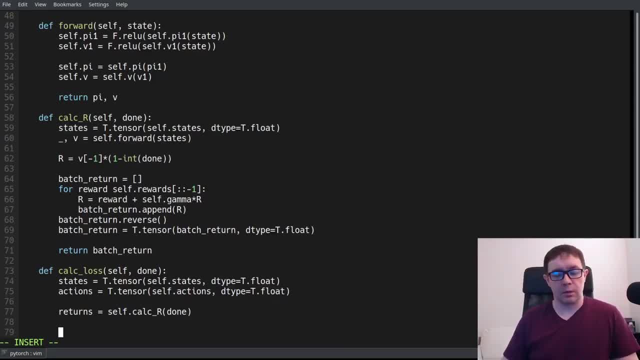 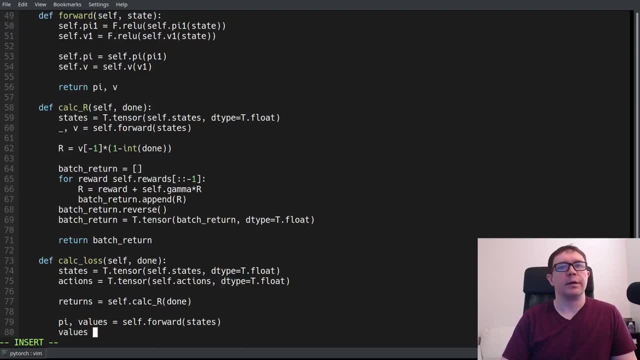 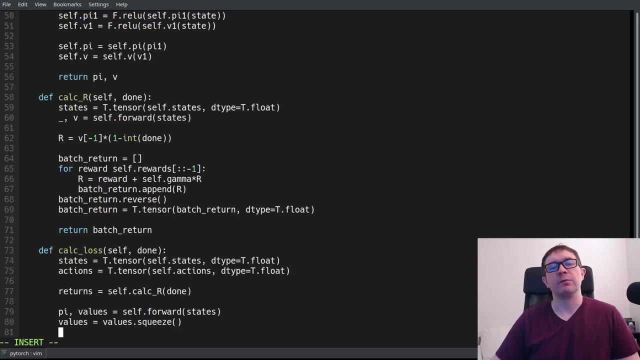 then we're going to use those quantities for our loss. functions, values, squeeze now. this squeeze is very important. if you don't squeeze here, it won't trigger an error, but it will give you the wrong answer. the reason it will do that is because the actor loss and the 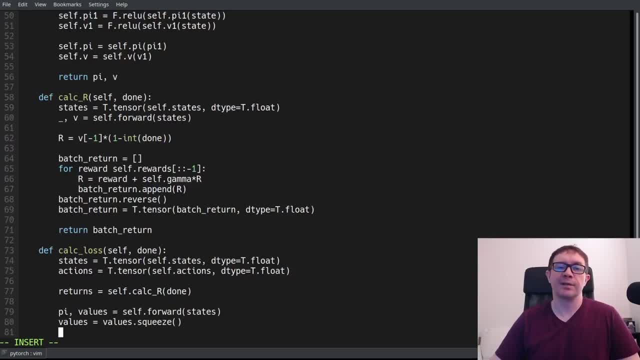 critic loss, i believe, will come out as shape five by five, and that is not the shape we want. we want something: in the case of five time steps, t max equals five, so it'll give you a five by five matrix and it'll give you a five by five matrix, and it'll give you a five by five matrix, and 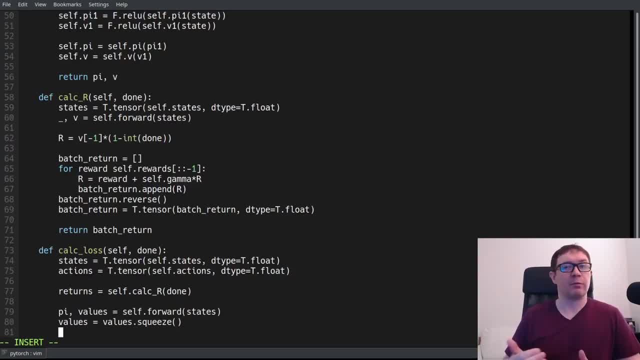 instead of a five element vector. so you have to perform the squeeze here to get the five by one output of the deep neural network into something that is just five: a list of five elements or a vector of five elements instead of five by one. so definitely need that squeeze if you don't believe. 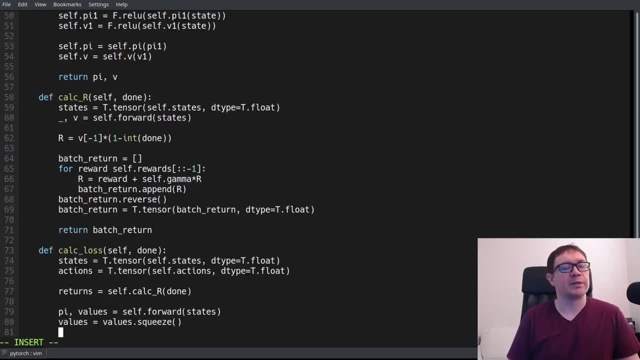 me. by all means erase the line or comment it out and print out the shapes of things to the terminal. i always recommend doing that. it's a good way of solidifying your understanding of how all this stuff works. again, our critic loss is just the returns minus values squared- pretty straightforward. 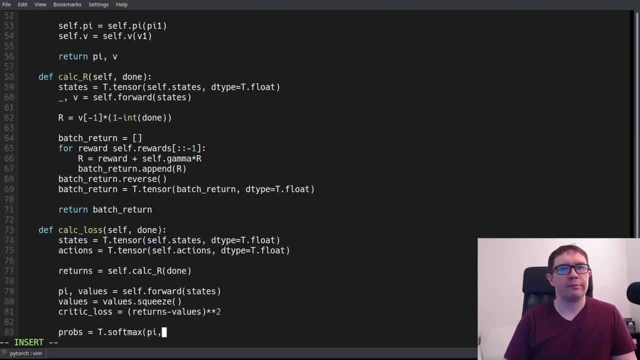 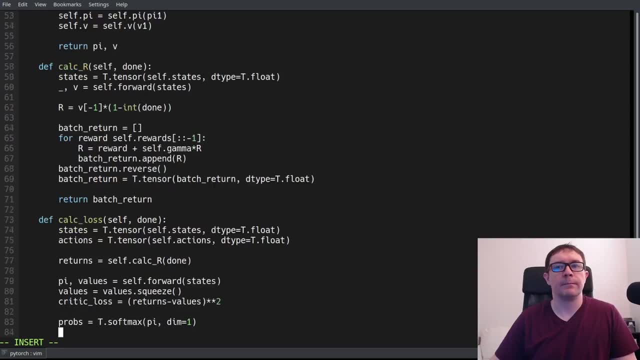 so now let's go ahead and say that we want the softmax activation of our output and that has a property that, of course, the softmax guarantees that every action has a finite value and that the value, the probabilities, add up to one, as all probability distributions, distributions should. so then we use that output to create a categorical distribution. 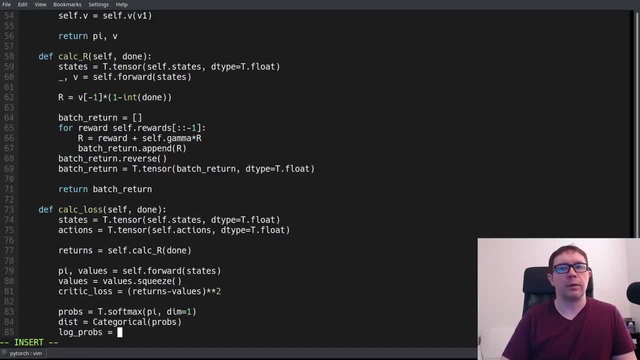 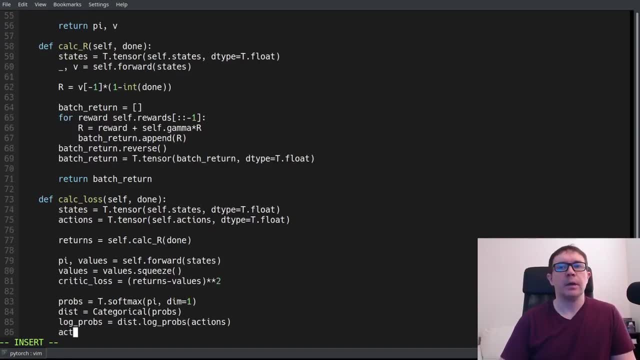 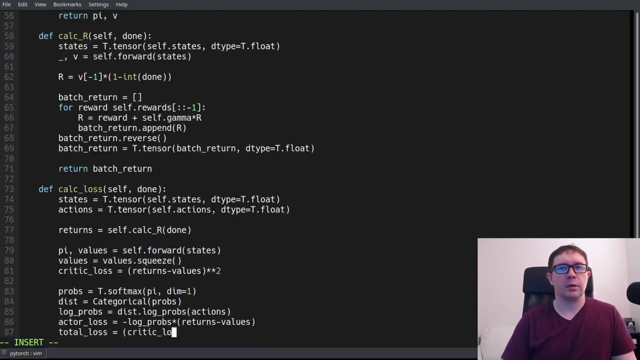 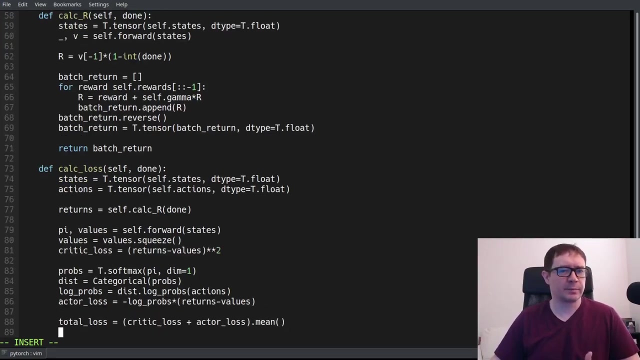 and calculate the log prob ability distribution of our actions actually taken, then our actor loss minus log probs times the quantity returns minus values. that's from the paper, And then our total loss is just critic loss plus actor loss. dot mean We have to sum the two together because of the way that the back propagation is handled by PyTorch. 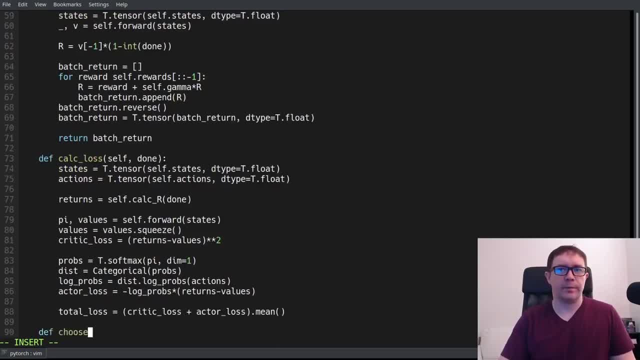 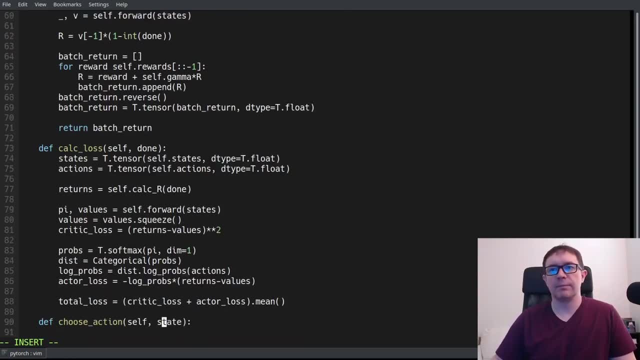 And of course I did forget to choose action function. but that is not a big deal, We'll just go ahead and handle that now. So that will take. we're going to call it observation as input, because we're going to be passing on the raw observation from our environment. 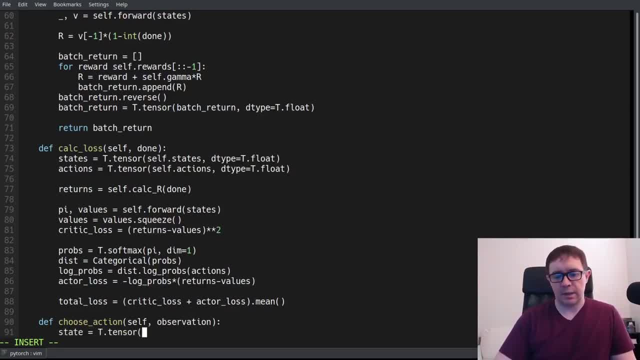 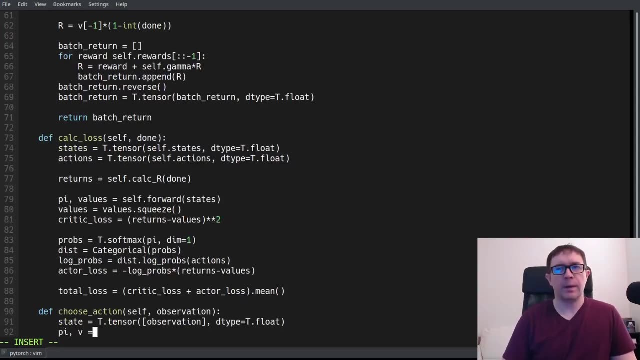 And so we have to convert that to a tensor right off the bat And we have to add a batch dimension to that for compatibility with the inputs of our deep neural network, And we're going to call it a D type of float. We pass that through our neural network. 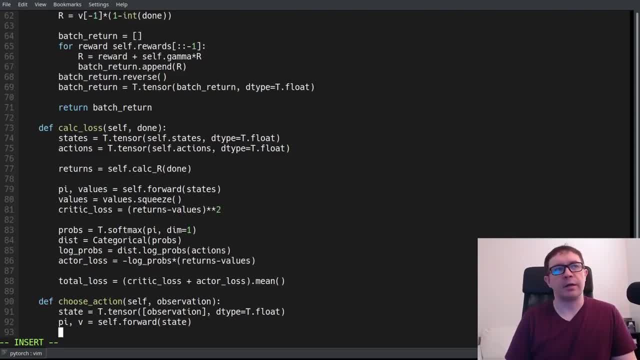 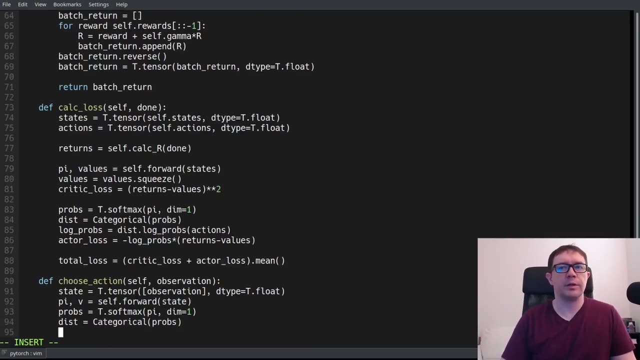 Get our policy and value function out, Perform a soft max activation on our policy along the first dimension. Then we're going to create our distribution based on those probabilities and sample it And convert it to a numpy quantity, Take the zeroth element and return it. 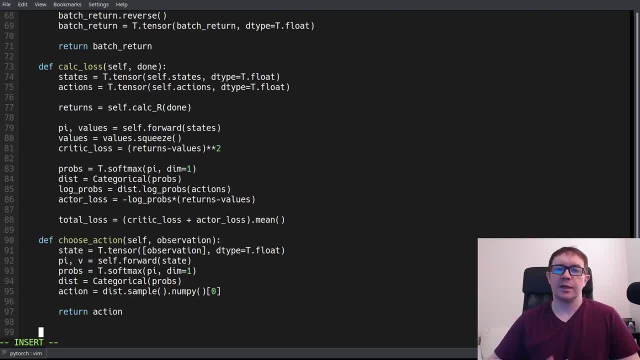 So that is it, And that's it for our actor network class. It encapsulates most of the functionality I would associate with the agent, But it does everything we're going to need each of the independent actors within their own thread to do. Now we're going to move on to the agent class that is going to handle our multiprocessing functionality. 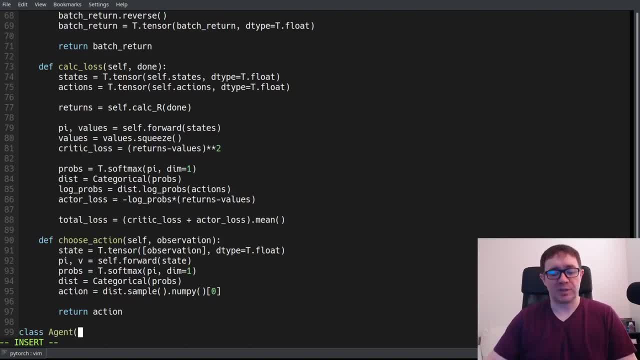 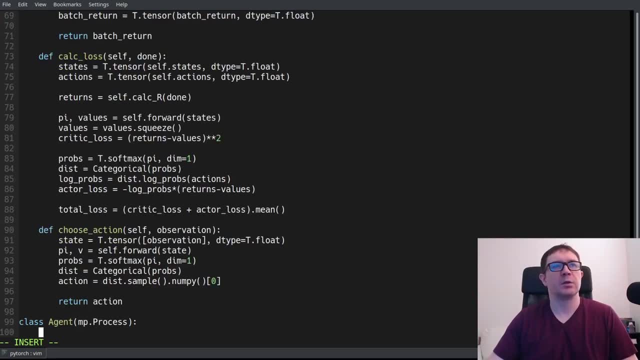 So I'm going to call this agent. You will sometimes see it referred to as worker and that is a fine name. That is kind of precisely what it is. I'm just using agent. to be consistent with my previous nomenclature, It has to derive from the NPTEL. 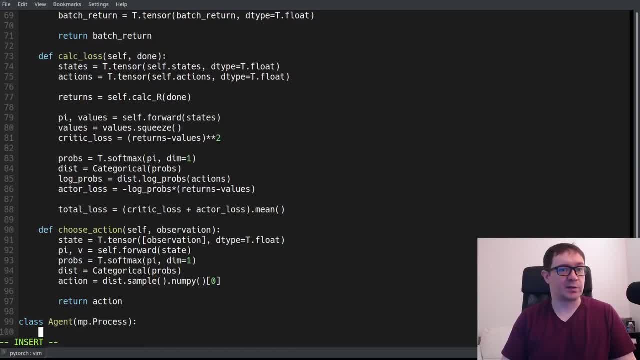 NP dot process class. So we get some access to some goodies there. So we will need our global actor critic. That is what is going to handle the functionality of keeping track of all the learning from all of our environment specific agents. The optimizer that is going to be the shared atom optimizer that we wrote earlier. 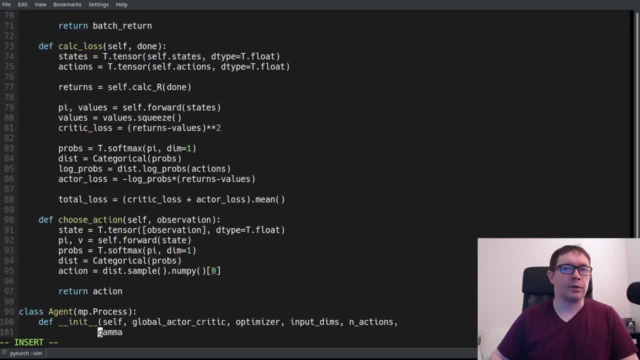 Input dims number of actions. Gamma, in case you want to use something other than 0.99, a learning rate, a name to keep track of each of the workers from our multiprocessing global episode index. So this will keep track of the total number of episodes run by all of our agents. 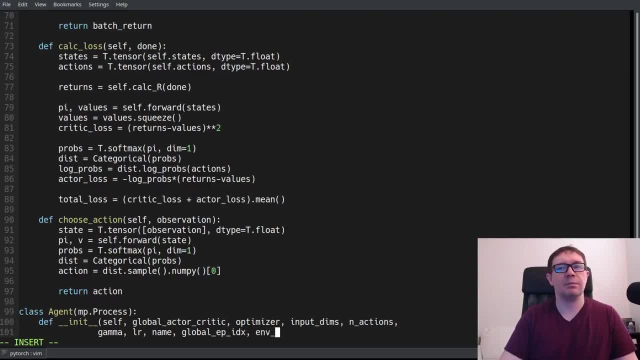 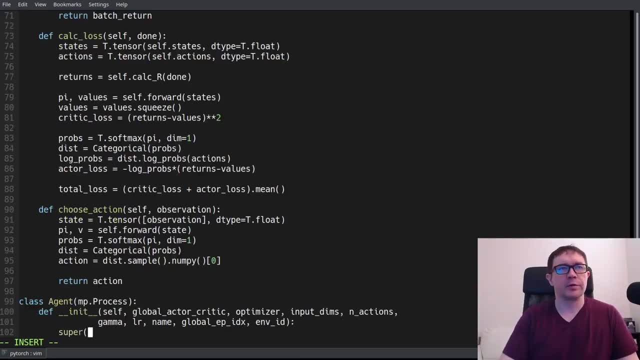 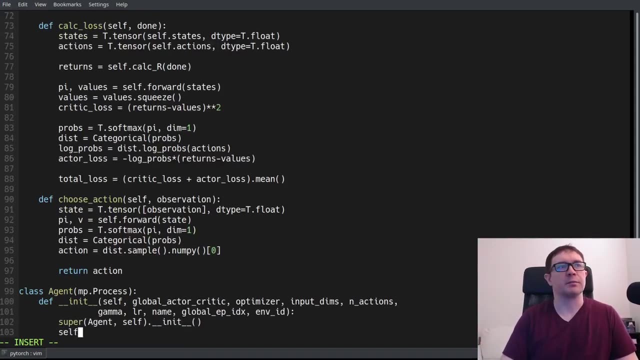 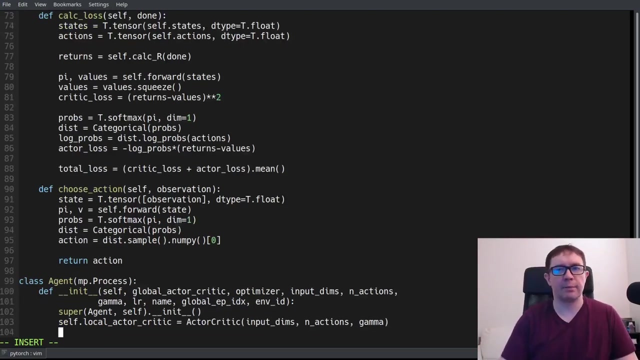 It's not as easy of a concept as it may seem, because you're doing asynchronous processing as well as an environment ID. So the first thing I'm going to do is call our super constructor And go ahead and start saving stuff. So our local actor critic is just going to be our new actor critic with inputs, of input dims, number of actions and gamma. 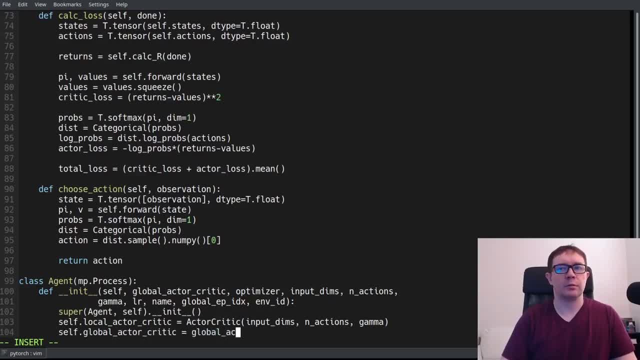 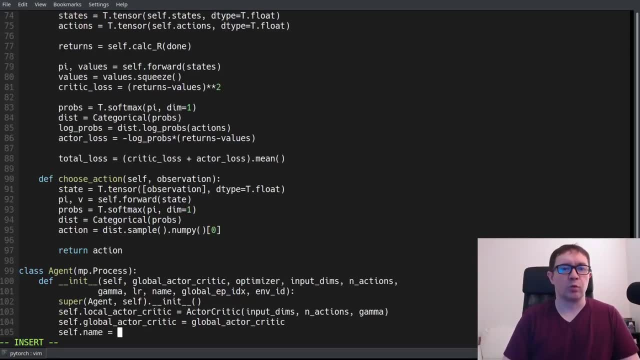 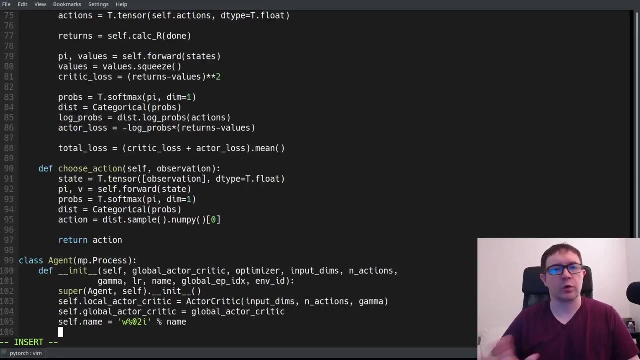 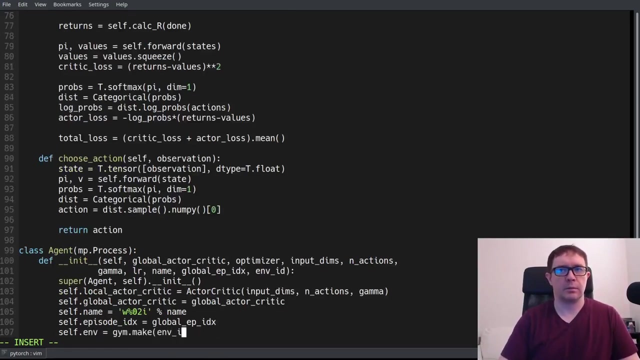 We want to save our global actor critic, we can update its parameters. we're gonna have a name for each worker in its own independent thread and that's just going to be just worker number name and then we'll have an episode index. well, what episode ID X? our environment. so 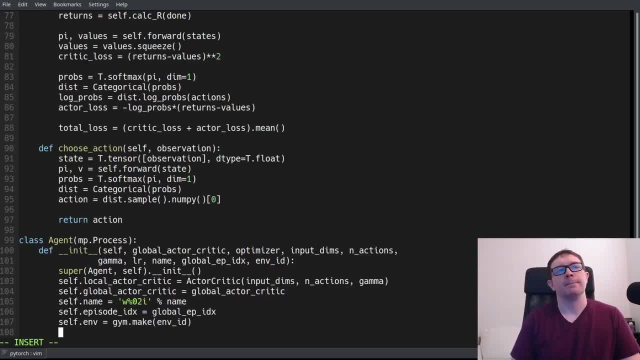 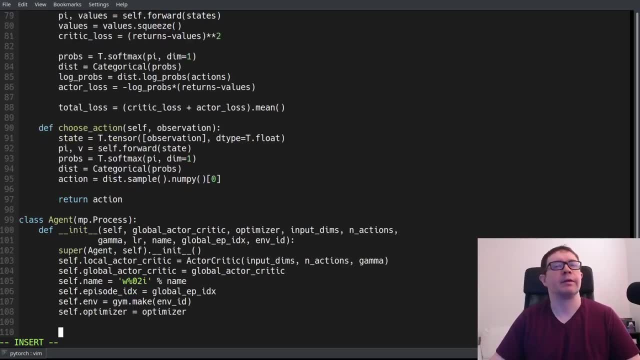 environment ID is a string here. that isn't clear and our optimizer. I spell that correctly. yes, I believe I did so. we have to define a very specific function so that stuff actually works, and that function is the run function. this gets called behind the scenes by the worker dot start function that we're gonna. 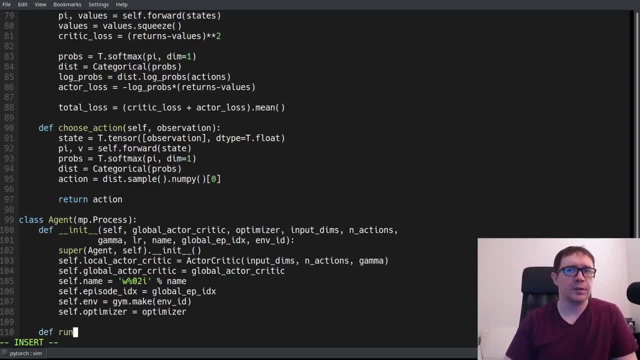 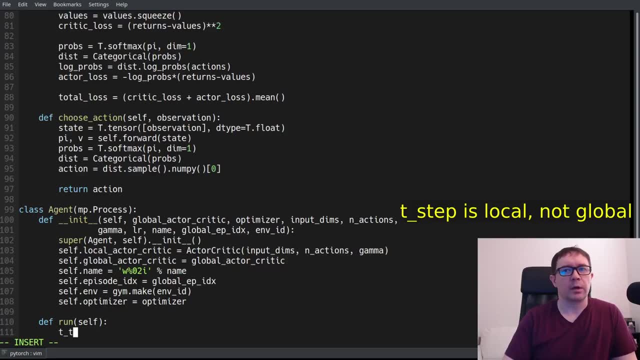 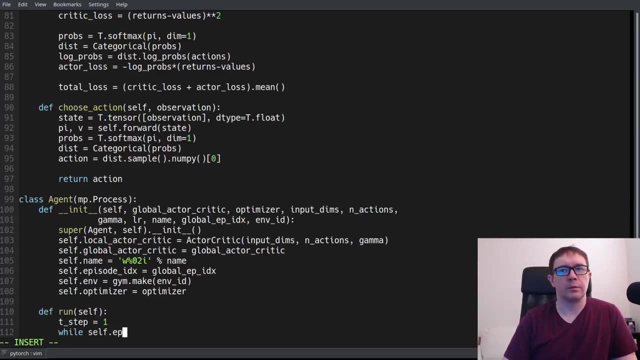 handle in the main loop, but this handles effectively all the main loop type functionality. you can see that we're gonna have a function that's gonna be called the of our problems. so our global time step is gonna get set to one, while our episode ID X value. so episode ID X is a global parameter from the multi. 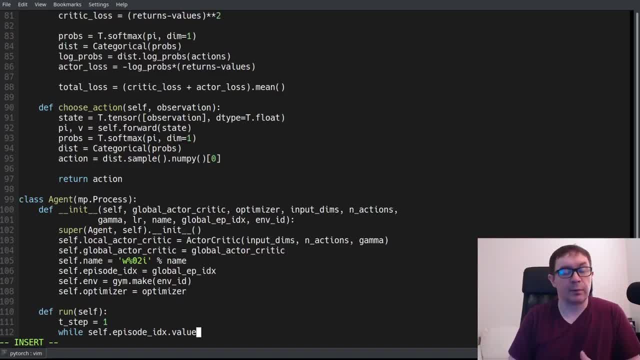 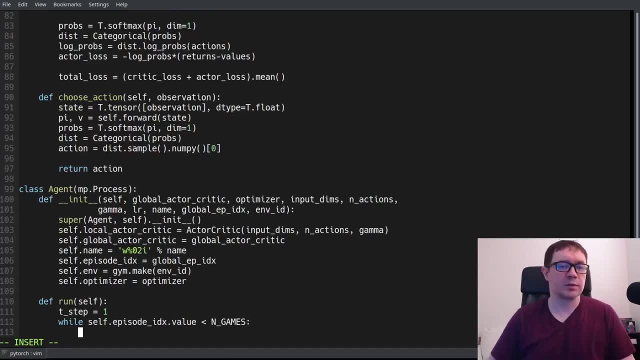 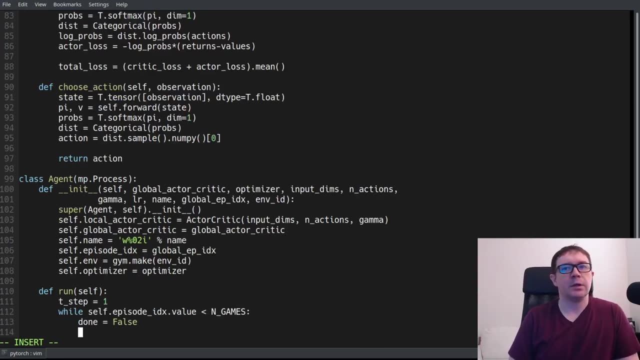 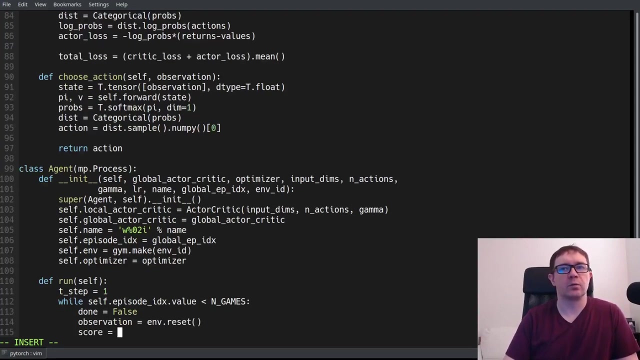 processing class and that we want to get the value by using the dot value D reference and, while that's less a number of games, some global variable we're gonna define. in other words, what? while we have not completed all of our games, set your terminal flag to false, reset your environment and set the score to zero. 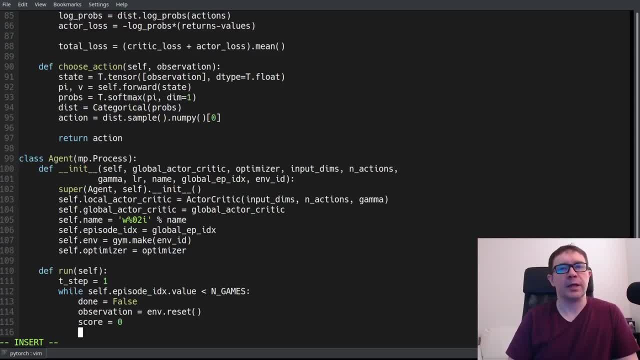 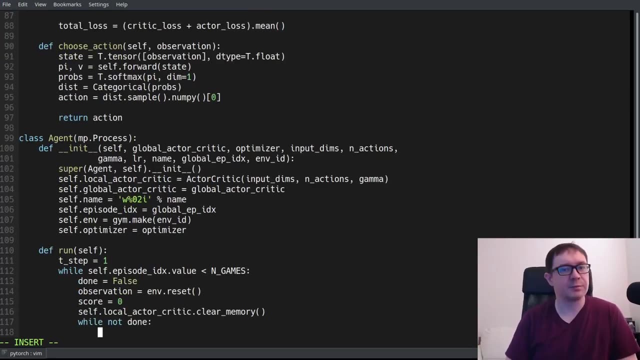 and go ahead and clear the agents memory at the top of every episode and then, while you're not done so, go ahead and play your sequence of episodes and see a- I'm sorry- sequence of steps. within an episode, the action is chosen by your local actor critic, so you're gonna pass the observation into each local actor. 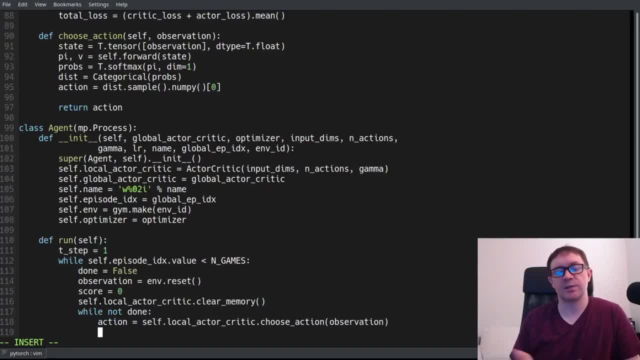 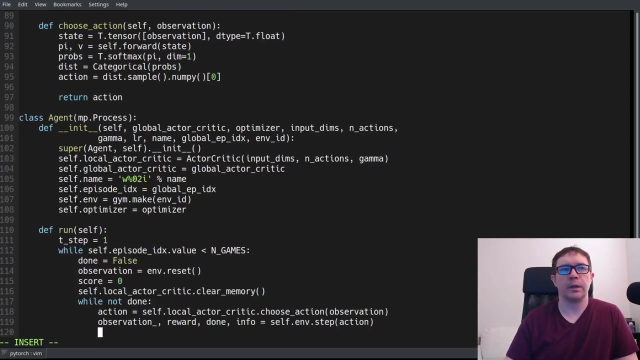 critic. so each of these 16- in this case threads will get its own local actor critic and that'll synchronize to the global. but you never actually use the global network directly to do things like choosing actions. so get the new state reward and debug info back from your environment. keep track. 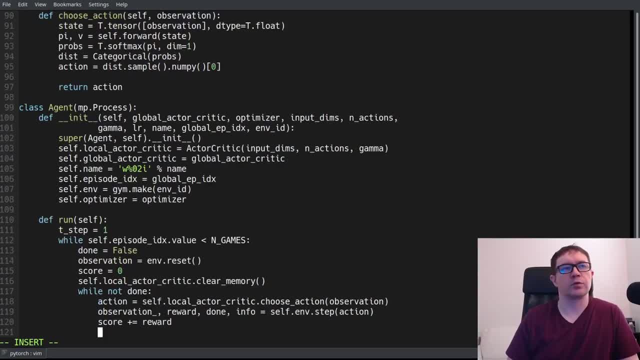 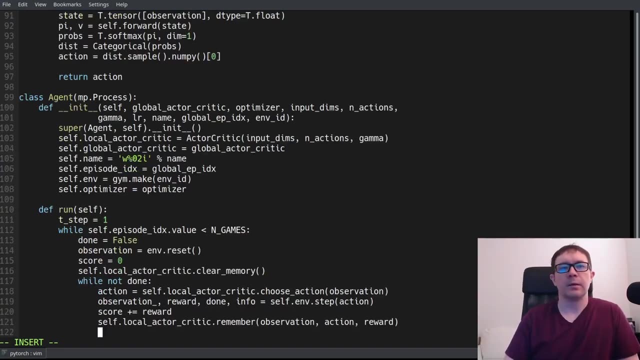 if other awards received as part of the total score remember that observation reward, then we have to say: If the number of steps modulus, the maximum number of steps is zero, in other words, if it is every fifth time step or we have finished the episode with that last time step, 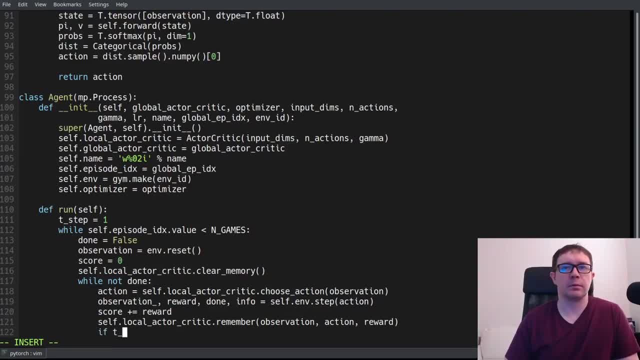 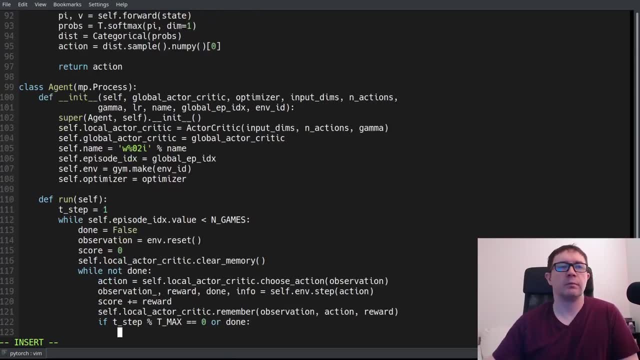 then we're going to go ahead and perform our learning step, Modulus T max. Well, we're done. Then we're going to go ahead and handle the learning functionality. So we'll say: loss equals local actor predictcalc loss. Of course we need the most recent terminal flag as the parameter for that function. the argument: 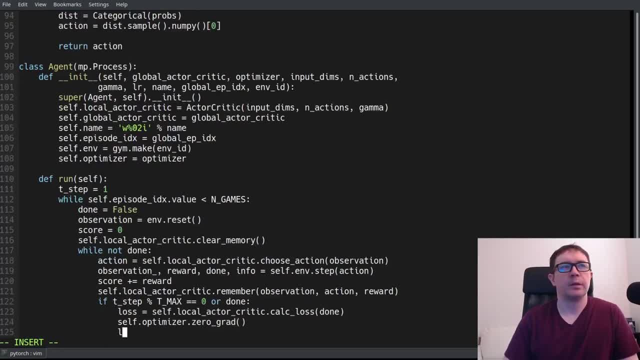 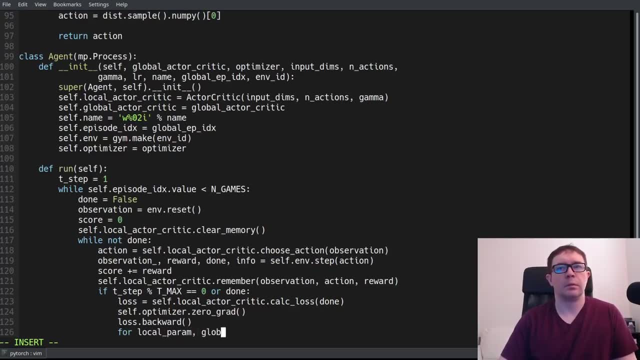 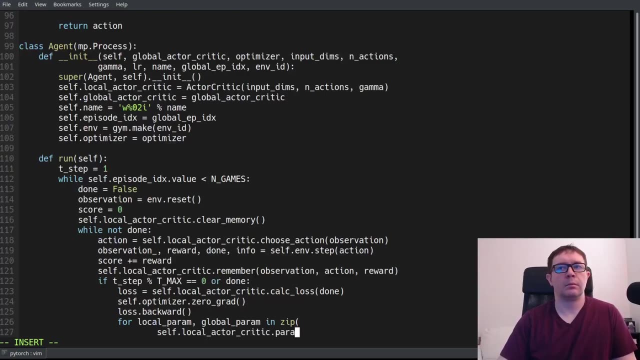 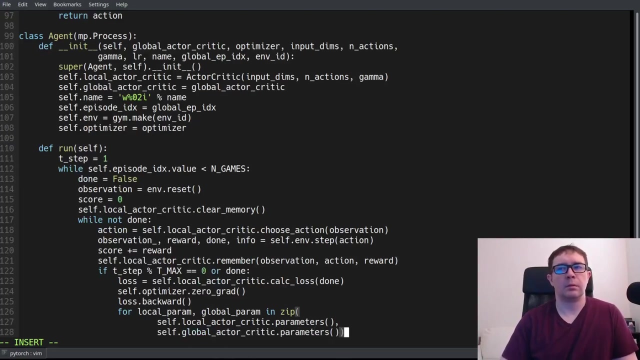 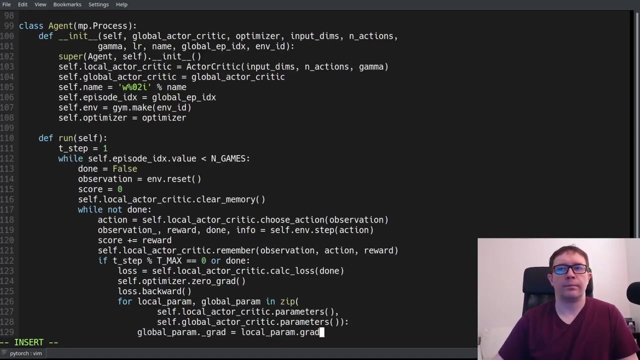 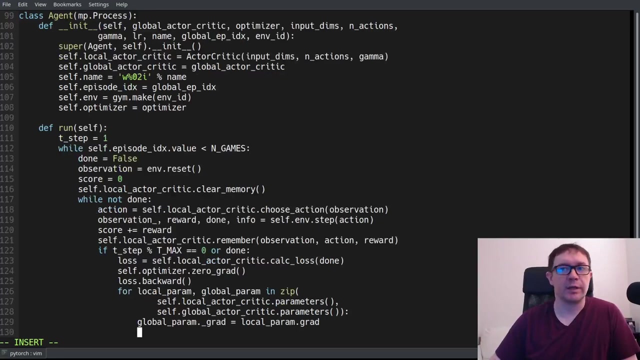 Go ahead and zero your gradient and back propagate your loss. So we're going to set the parameter for the global gradient to the local agent's gradient at this step And then, after doing that, we can tell, we can tell our optimizer to step. 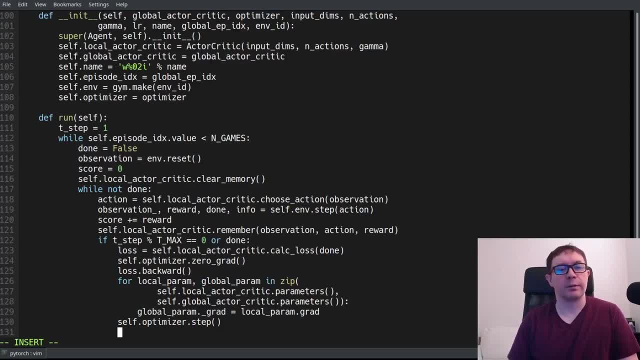 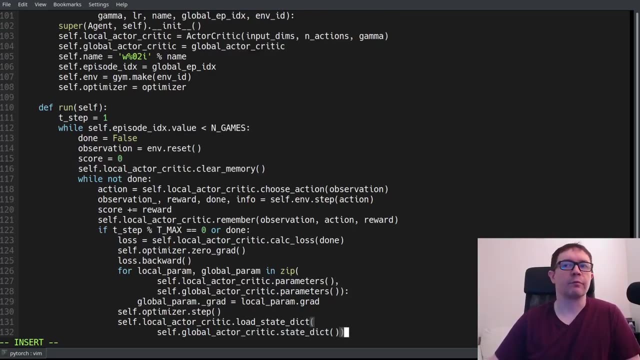 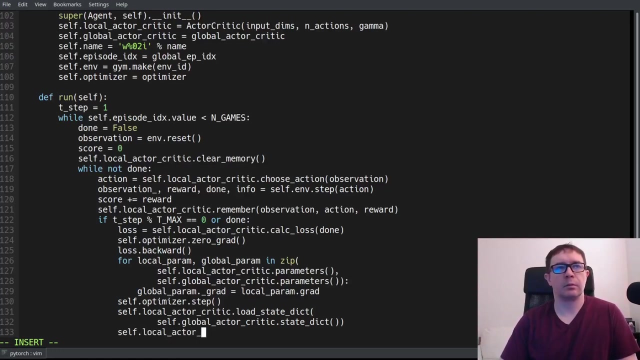 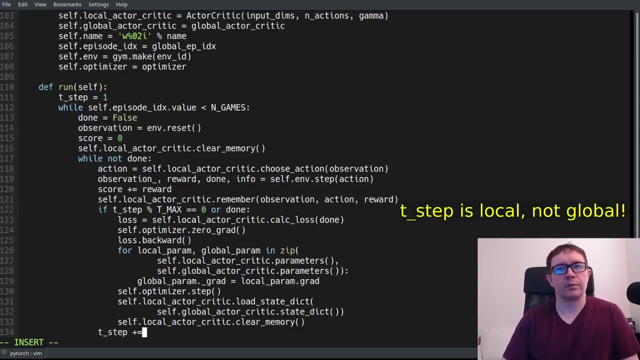 And then we can go ahead and synchronize our networks, And we do that by loading the state dictionary from our global actor critic to our local one. And then we want to go ahead and clear the memory After each learning step and then tell the algorithm to increment T step by one. 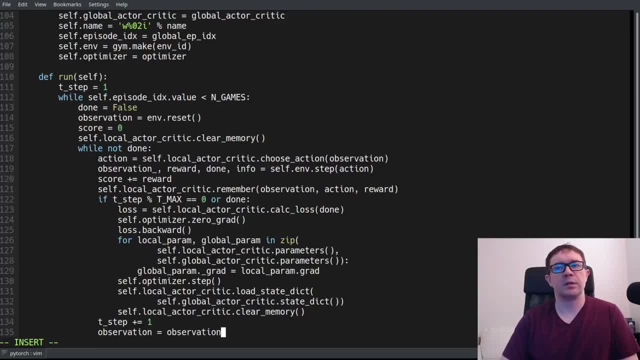 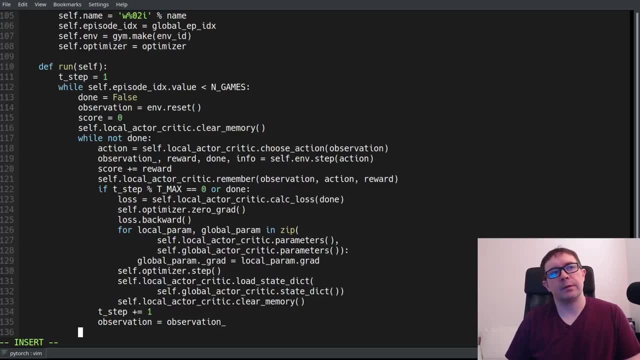 the global time step and set the current state to the new state. Then at the end of every episode we have to handle the, the fact that we may have finished an episode from another agent while one- Fred- was running, because this is running asynchronous, asynchronously. 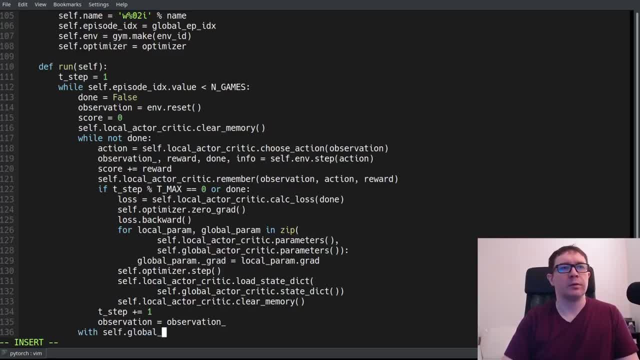 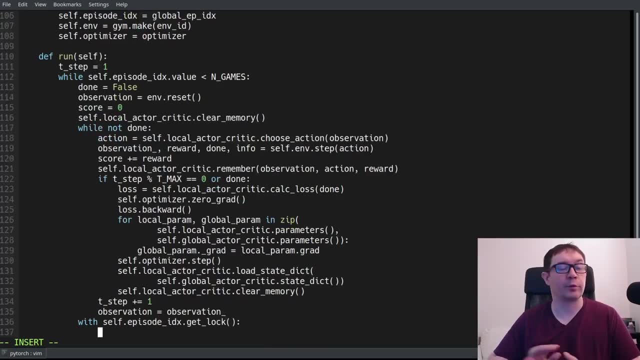 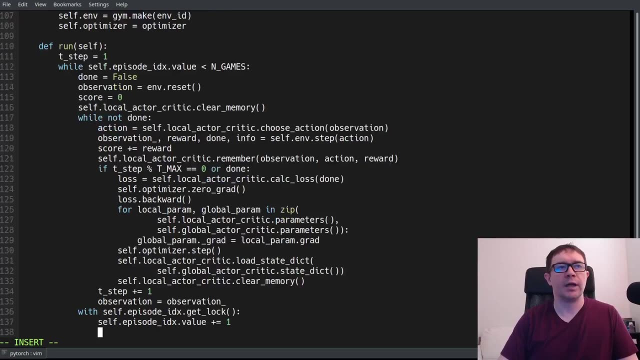 So we say with selfcom global- sorry, selfepisode IDX dot get lock. So we want to make sure that no other thread is trying to access that variable right now And if we can go ahead and increment that episode value by one. 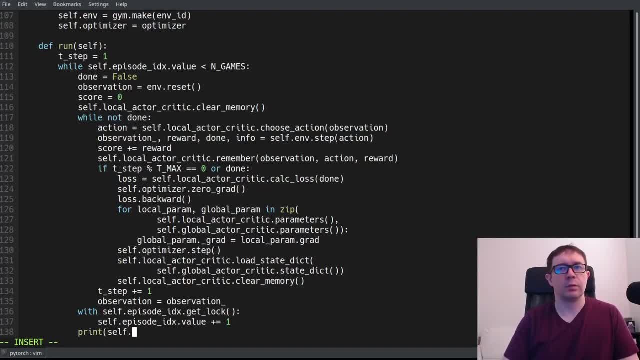 then we do the usual print the debug stuff to the terminal. We're going to print out the name of the worker, the episode, And that is selfepisode, IDX value and the reward, the total score from the episode. And that is it for our agent class. 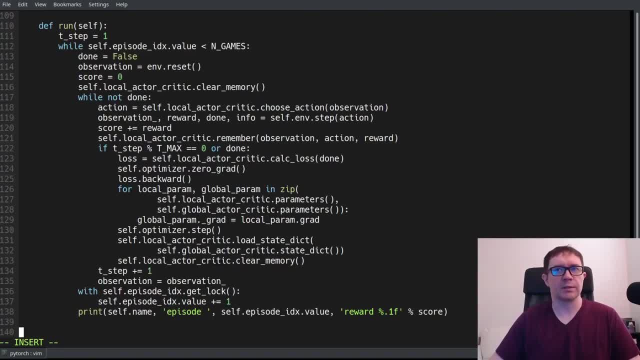 So this is relatively straightforward. All we're doing is now handling the fact that we have our local parameter, our local agent that chooses actions. We're going to perform the gradient descent, optimize or update using the gradients calculated by the actions of that agent. 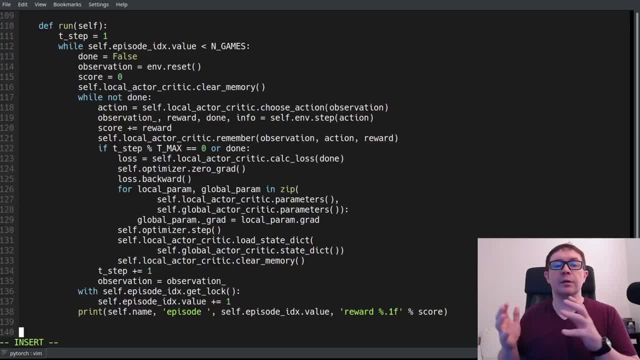 and then upload that to our global network, so that every, every agent uploads its learnings to the global network. And then we're going to go ahead and download that from our global network as well, so that we make each agent in its own thread better over time. 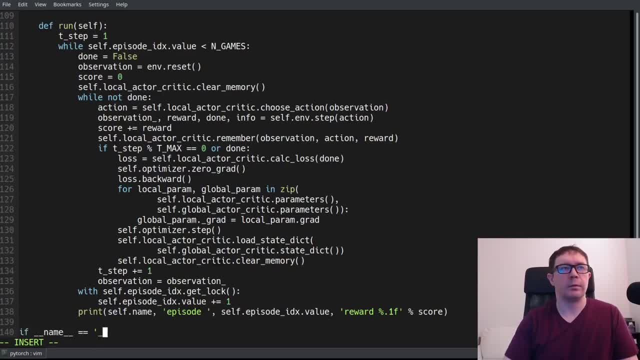 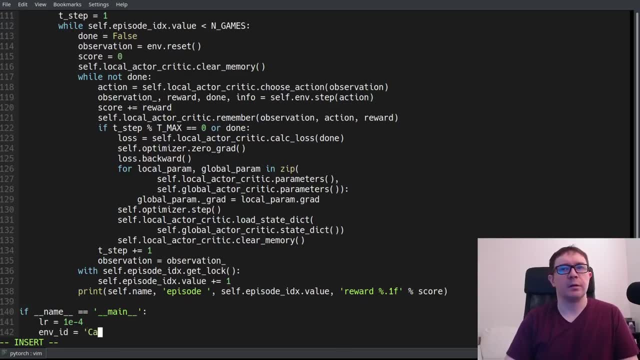 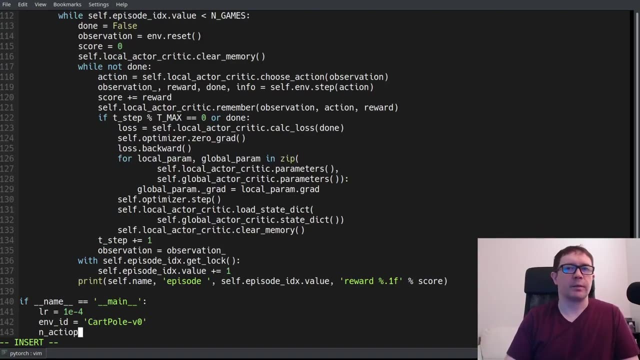 Now we have our main loop and we're going to do some stuff like declaring our learning rate, our environment, ID cart pole V: zero. number of actions for that environment is just two left and right Input. dims is just a four vector. 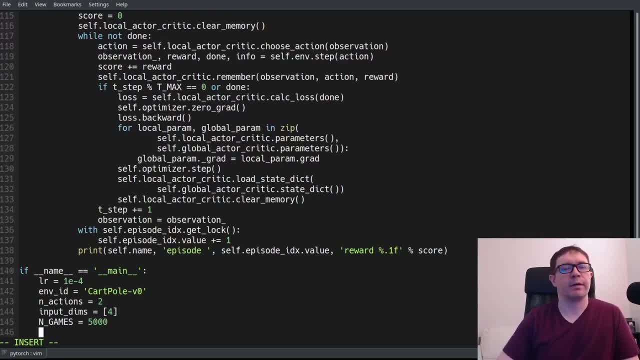 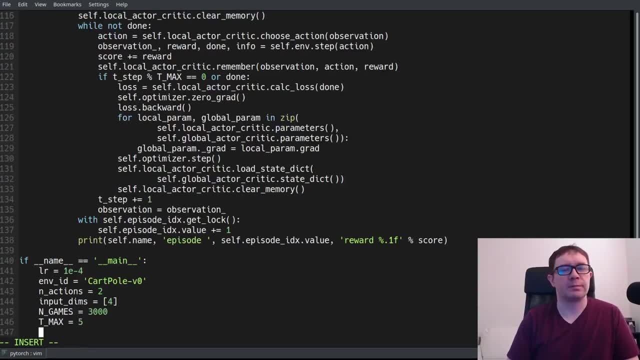 Uh, we'll say number of games by thousand. you know we can actually get away with 3000, I believe a team max every five steps. that comes from the paper. a global actor critic gets initialized here and that takes into dims and number of actions. 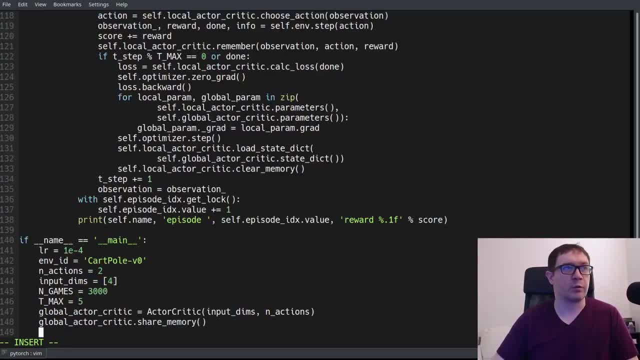 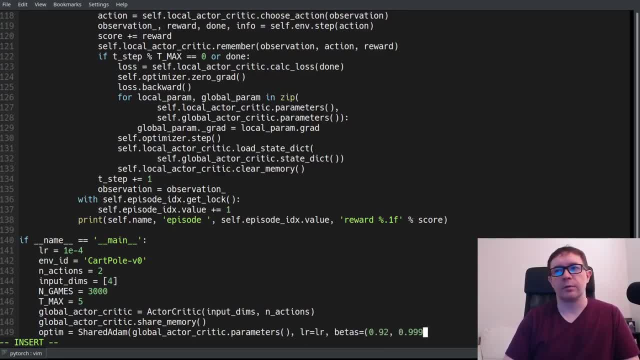 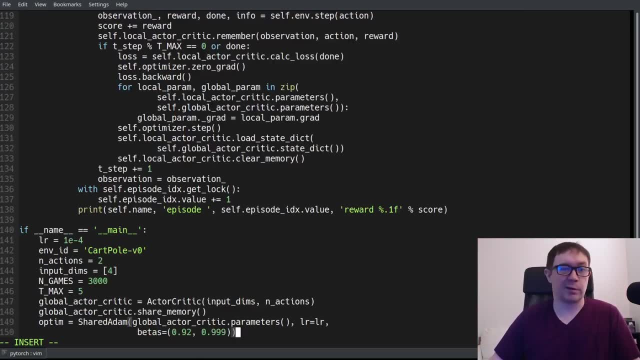 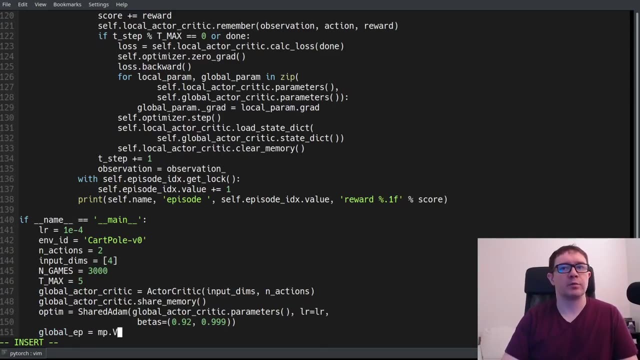 uh, uh, uh, uh. 0.920999.. I get that from more Van Joe's stuff. Uh, I haven't experimented with that too much. A little bit of cargo, cargo called programming here. I apologize for that. Now we have our global episode and that is just going to be a value of type. 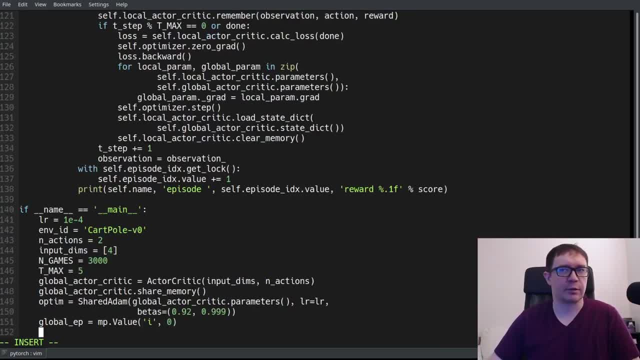 I. that means unsigned integer, doesn't mean I as an encounter variable. You could also have a D for a double if you wanted to keep track of like a score or something like that. I just means unsigned integer or no, it's a. 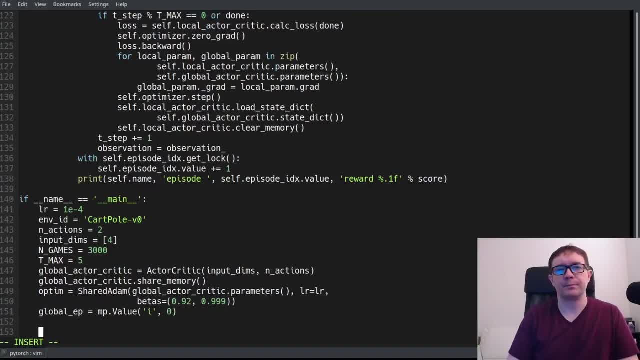 it's a sign in the term, So it can be negative as well as positive. Now we have to create a list of workers, and that's going to be a list of our agents, And this is what's. this is the construct that we're going to use to handle the. 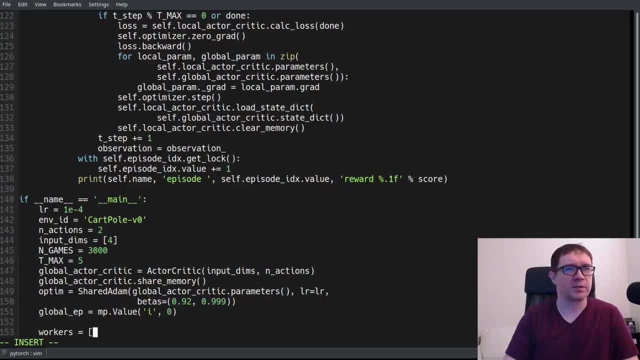 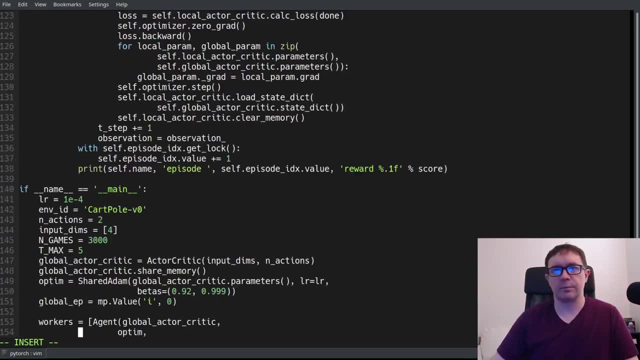 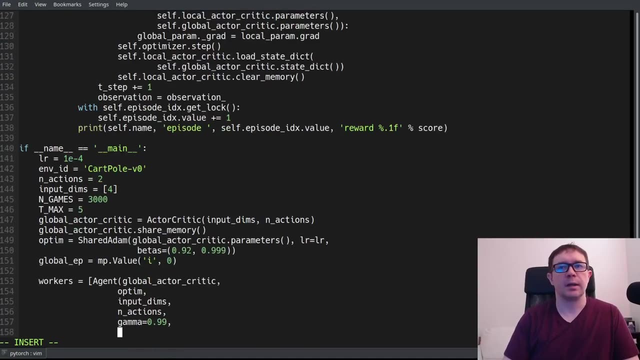 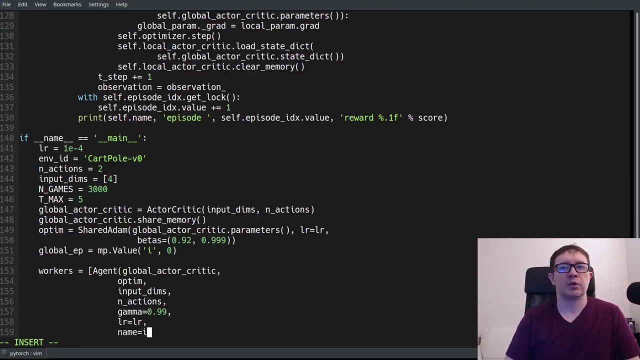 um, starting and running of our specific threads. So that's an agent We have to pass on our global actor, critic or optimizer. Our input: DIMS: number of actions, a gamma learning rate. It's helpful to use commas. Our name is just going to be the. 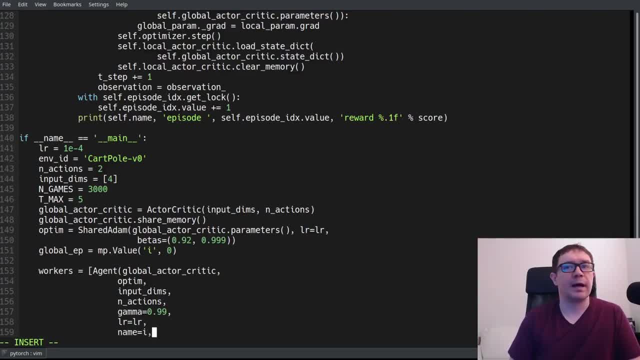 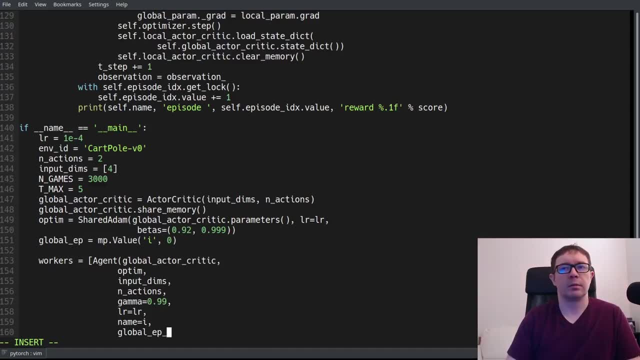 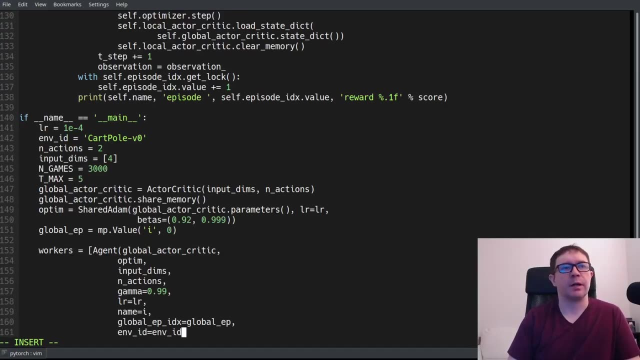 um, the name is just going to be the uh I in our list comprehension, our global episode IDX is going to be that global EP variable We just defined and we're going to pass in our environment ID or I in range. 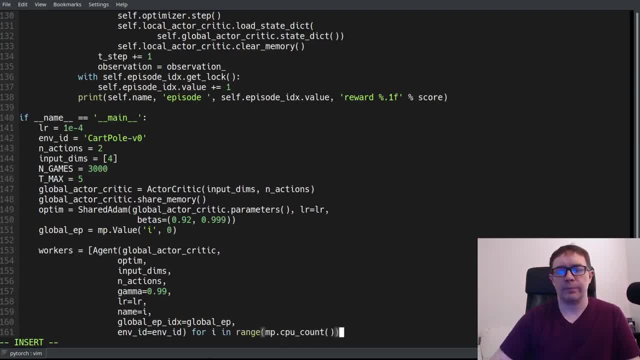 multiprocessing that CPU count. Now I haven't noticed a huge difference in uh running this with different numbers. So something other than CPU count and the range: I have 16 threads. If I tell it eight, it still uses all 16.. 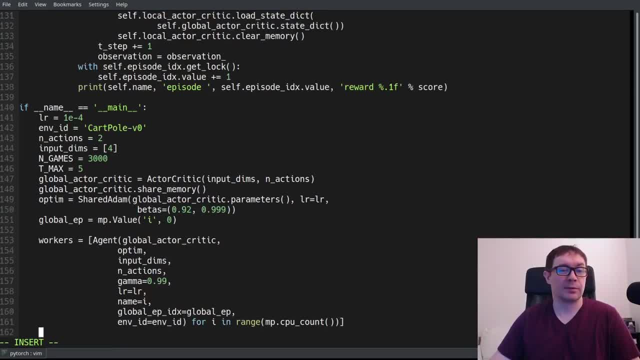 So I'm probably missing something here. Uh, I could do a deeper dive into the documentation to figure it out. Uh, but for the purposes of the video, I'm just going to go ahead and roll with it. So now we want to go ahead and start all of our workers. 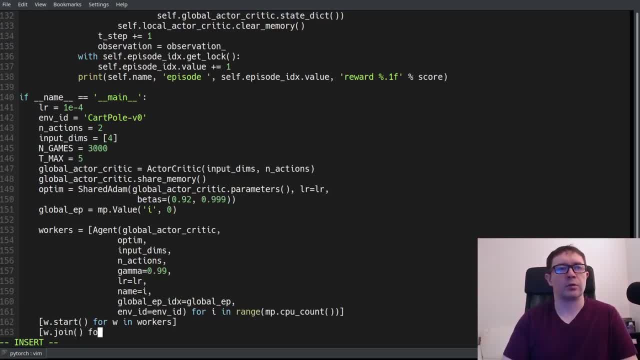 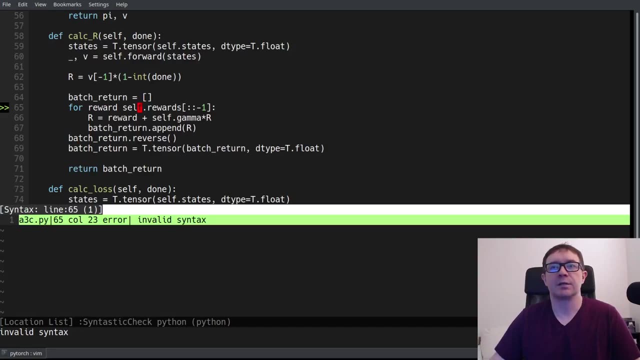 and then go ahead and do our joint operation. Okay, so now, moment of truth. I want to find out how many typos I made in the recording of this. Let's go ahead and do a right quit. I already have an invalid syntax. 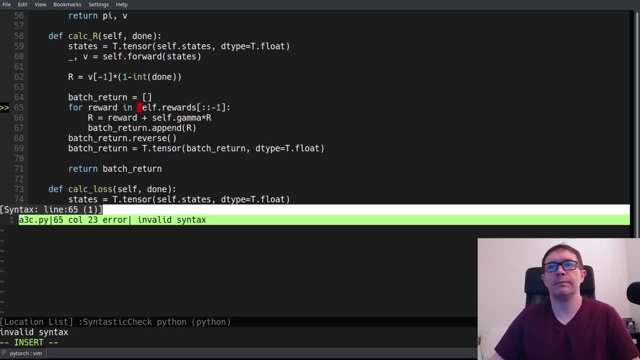 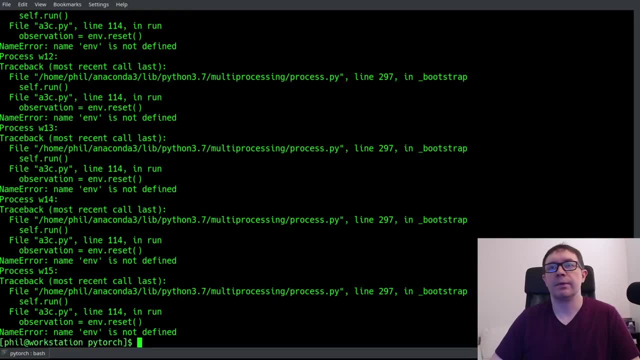 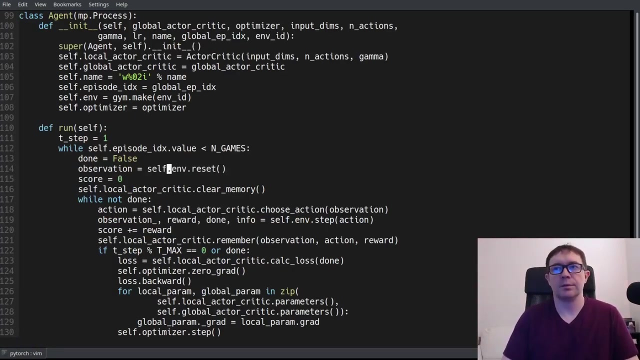 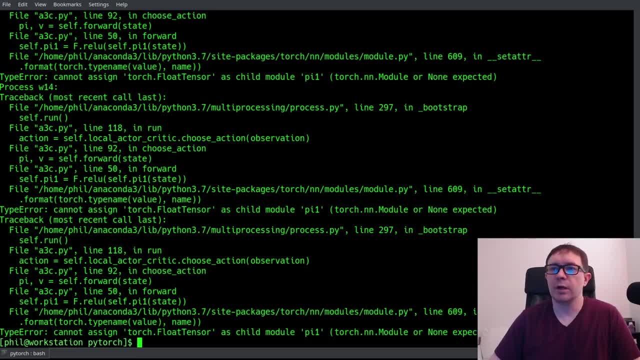 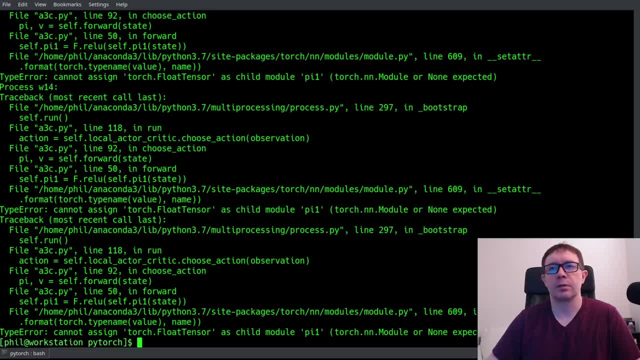 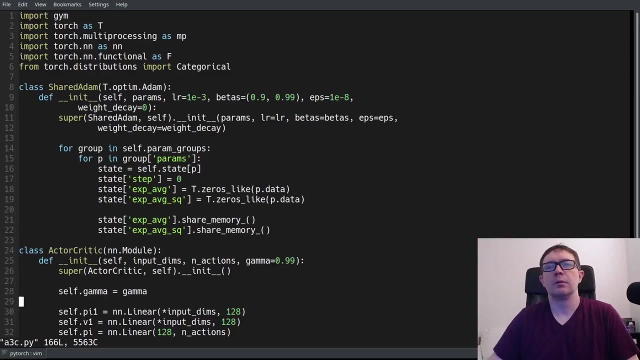 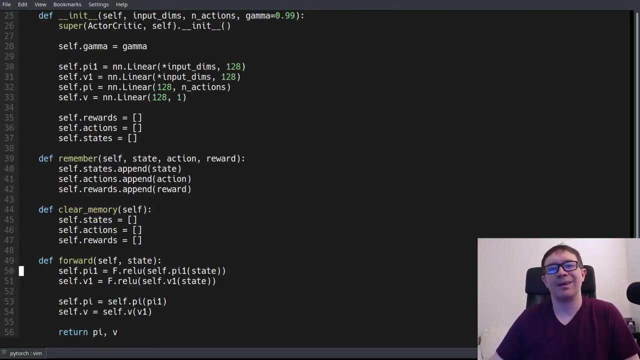 So that is when I handle the feed forward in our choose action function. Ooh, this is an interesting one. I haven't encountered this before. Let's take a look. Cannot assign as child module PI one. Oh, It's because, oh, of course. yeah, obviously I don't want that self here ought to annotate that. 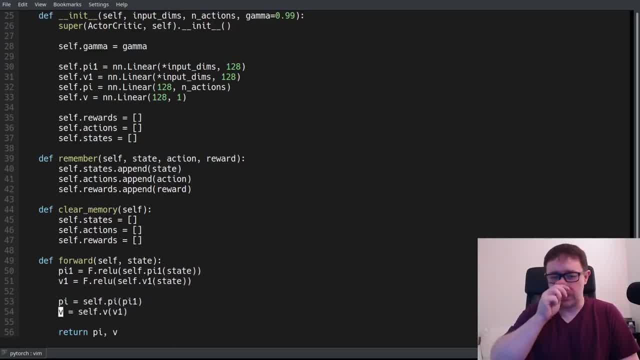 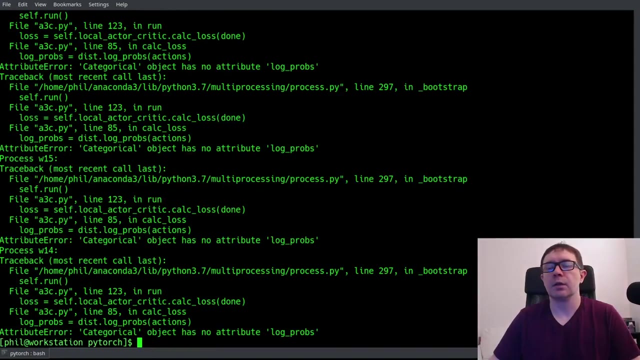 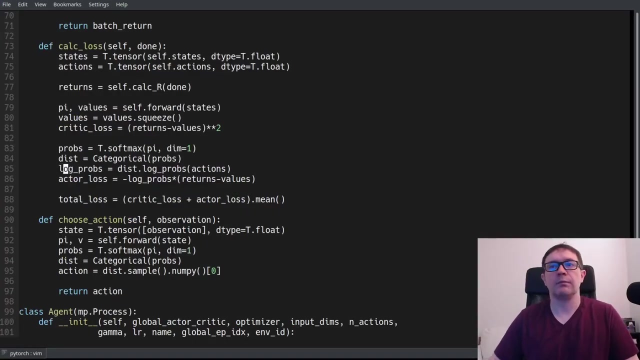 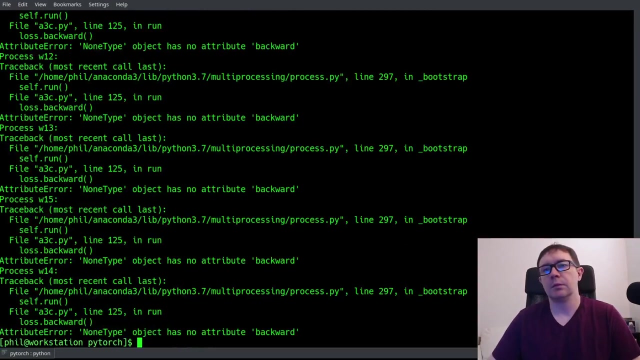 when I am editing the video. that is obviously going to be problematic. so you'll probably have seen that already that I put in a no self dot in there. okay, that's the beauty of doing things. for oh, it's because it's log prob, not log probs, that's in 85 problem. I hope I remember all these. there's none type. 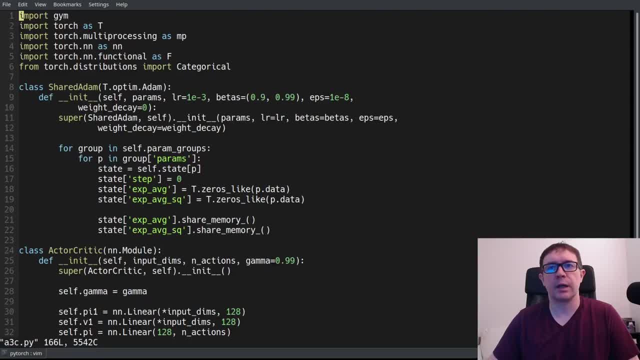 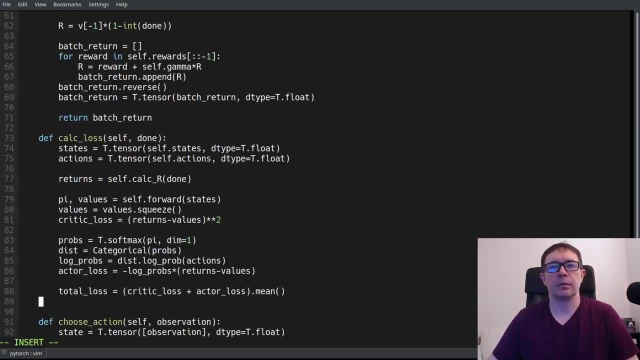 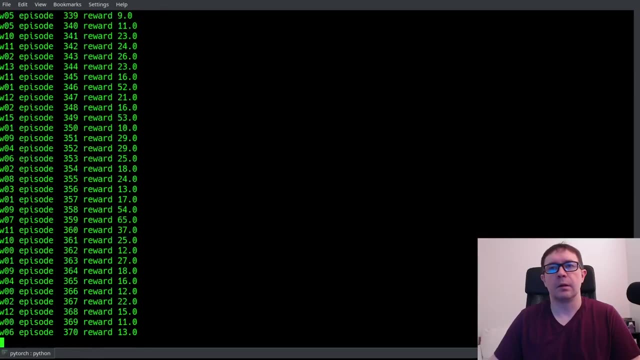 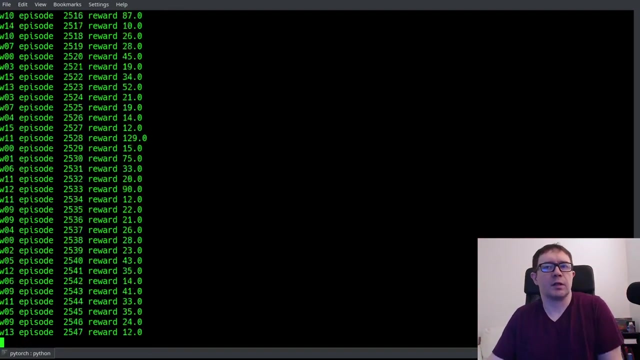 object has no attribute backward. I probably forgot to return you my loss. yeah, that's right there. we go all right. now it's running. hopefully it's still going to record, even though it is running across. all of our threads looks like we're still good now. you see, that executed really, really fast it was. 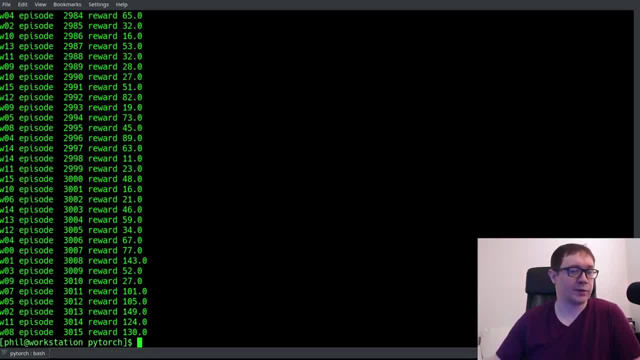 so fast. I didn't have time to get up the thread count, the resource monitor, to show you guys how to do that. so I'm going to go ahead and go ahead and submit it and let's see, guys. but you can see here that it achieves a non-negligible score. that. 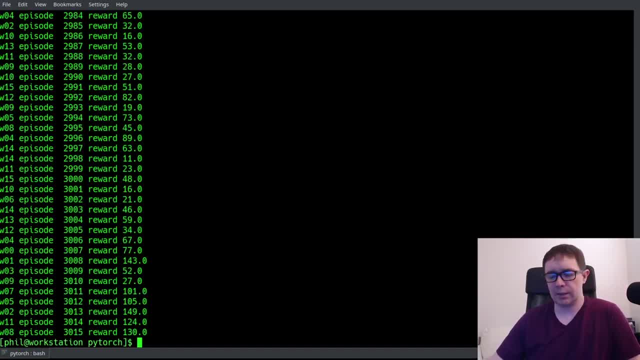 indicates some learning is going on. now let's go ahead and run it again and you can see now, this time it's not doing any learning at all. so there is a amount of run to run variation. so I'll let it run and finish and we'll try one. 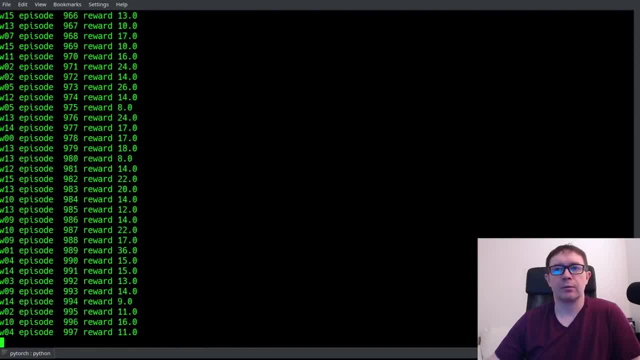 more time and maybe we'll get lucky and it will actually approach a score of 200. we defined some entries, we have 20, many numbers and we describe different limins. so I can just take a look here out of the window and type in conditions. obviously one milestone data as a sulky question: how much time we get for loved. we also have an indicator here to study data for aіз. Do we wanna know how tear minutes good for you guys? but yes, in this short video I am going to copy this and shut thisough roadhouse health. I'm going to talk to see how bad it is at another point. 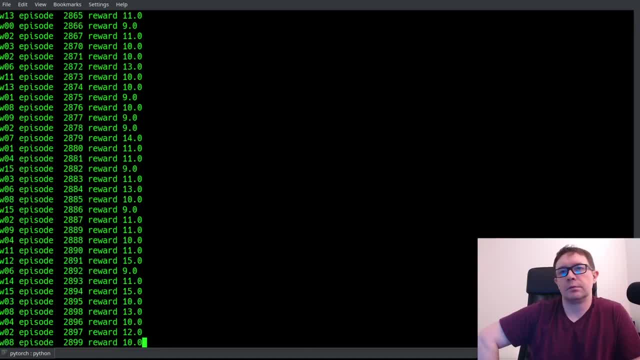 score of 200.. Now, that's one of my big criticisms of this algorithm is that there is a significant amount of run-to-run variation and it is pretty brittle with respect to some other algorithms that came later. Basically, the main advantage here is that it's asynchronous and this paradigm can be.